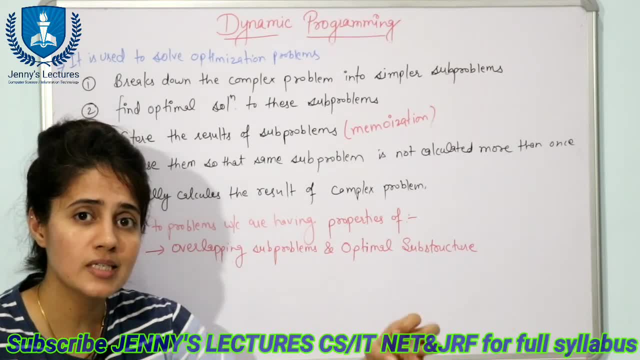 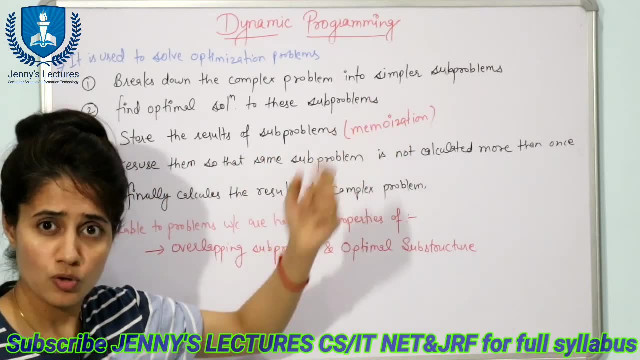 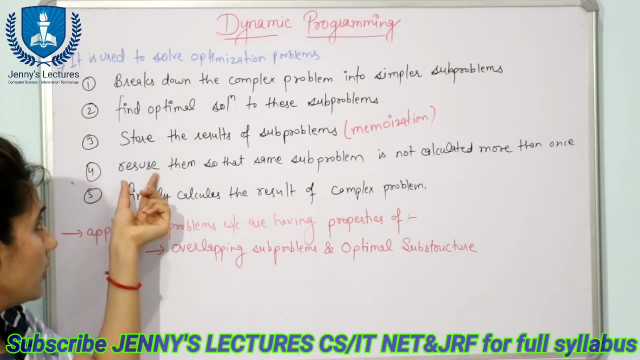 solution for these sub problems. Find optimal solution for these sub problems. Third point is store the result of the sub problems You are finding. you are finding out optimal solution of sub problems, plus, you are storing that result, Fine. and next point is reuse that result of sub. 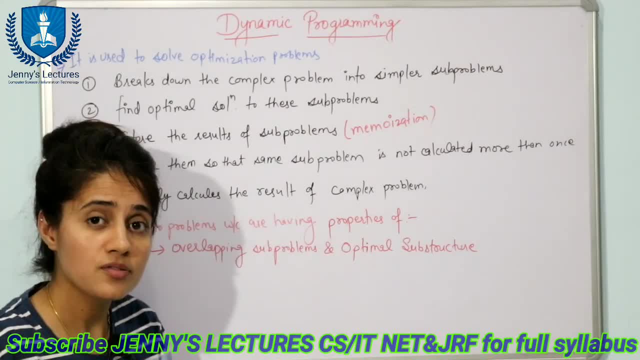 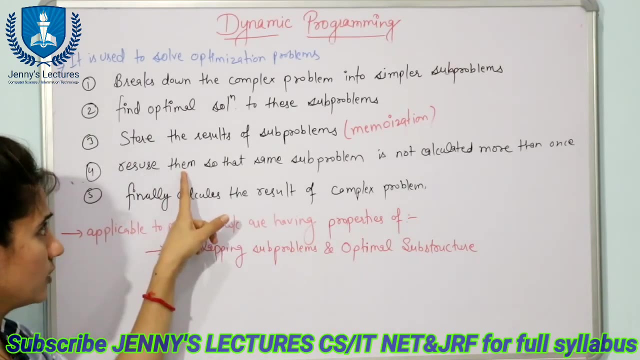 problems and why we are reusing that result, So that if same sub problem comes, then you you don't have to recompute that sub problem. That sub problem you just check out, you are having the result of that sub problem and you can take out that result. Fine, so reuse the result, so that same. 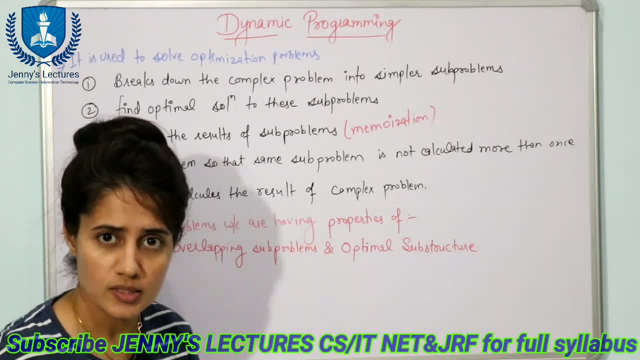 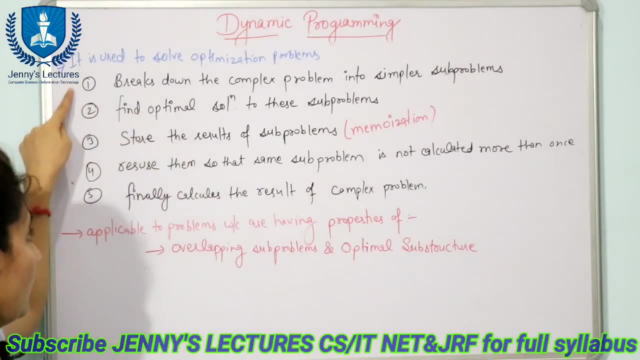 sub problem is not calculated more than once. Fine, and the final is finally calculates the result of complex problem. So these are five basic problems of complex problems. Now I have given you the are five basic steps of dynamic programming, how to use dynamic programming, and plus this, this is: 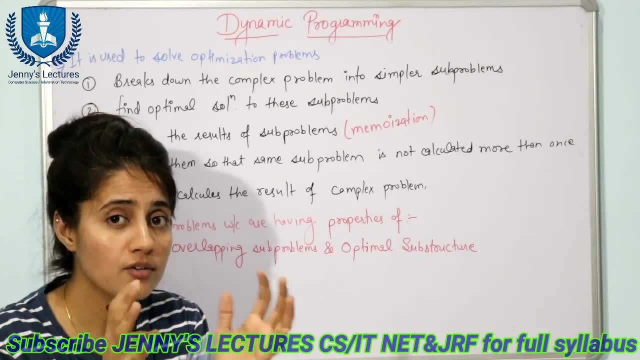 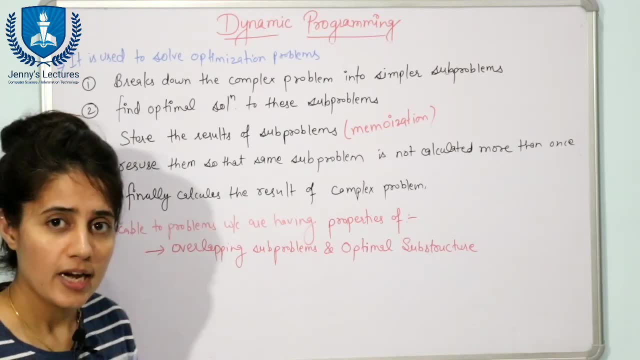 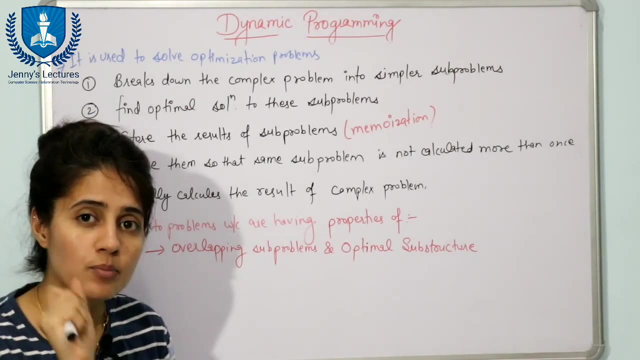 storing of the intermediate result, or you can say storing of that result of sub problems, is known as what memoization. so here one more point is there. see dynamic programming approach basically is used to solve or is applicable to the problems which are having certain properties, and those properties 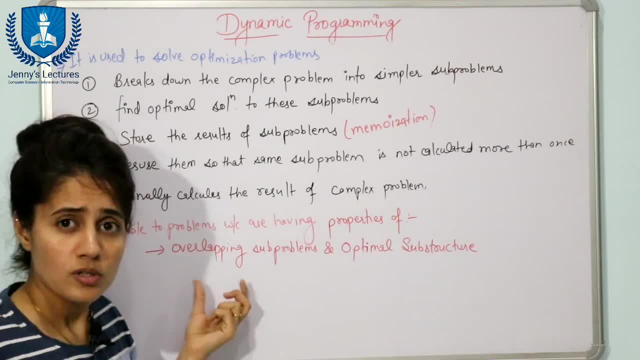 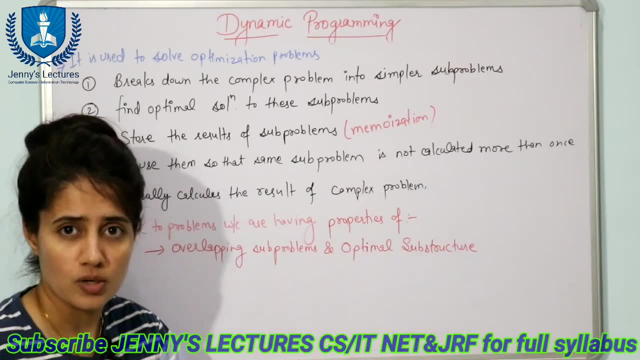 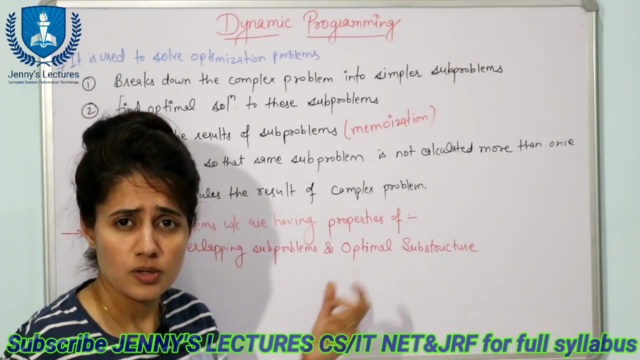 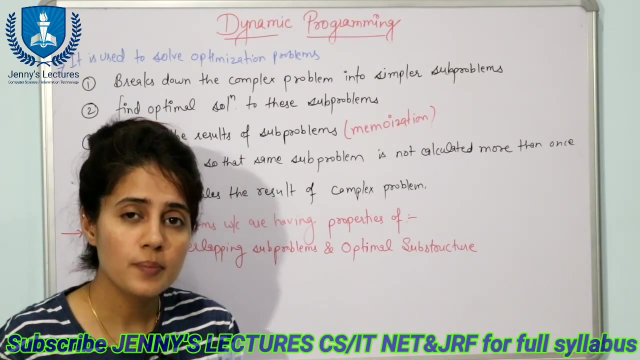 are the basic or the main properties? are those those problems should have properties of overlapping sub problems and optimal substructure. fine, we will discuss what is this overlapping sub problems- with the help of one example. see this: optimal substructure means the solution of a given optimization problem can be obtained by combination of the optimal solutions of its. 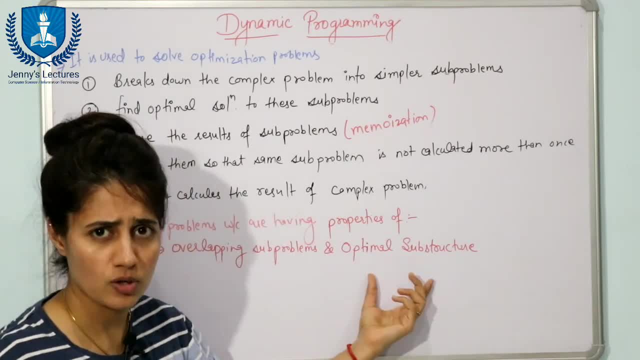 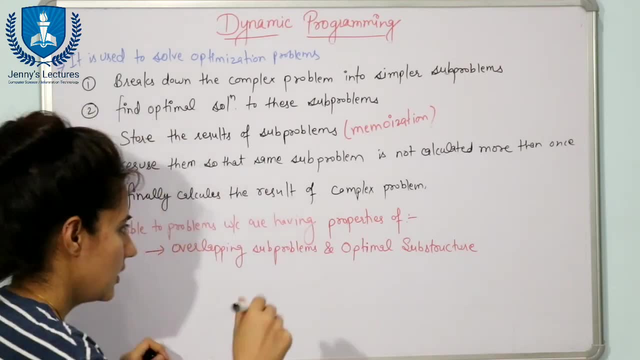 sub problems. that is basically you can see here, known as optimal substructure, and this we will going to discuss in with help of an example. so let us take one example. see, suppose I am writing here 1 plus 1, ok, and now suppose we know this one. 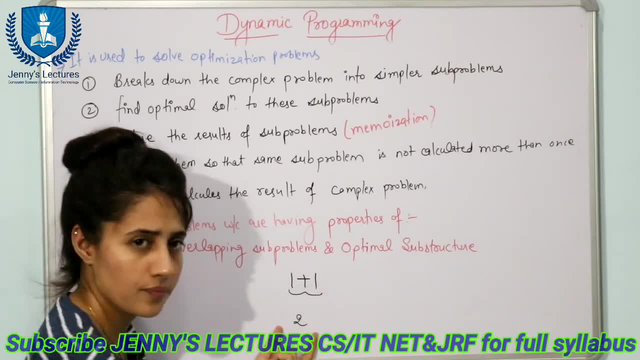 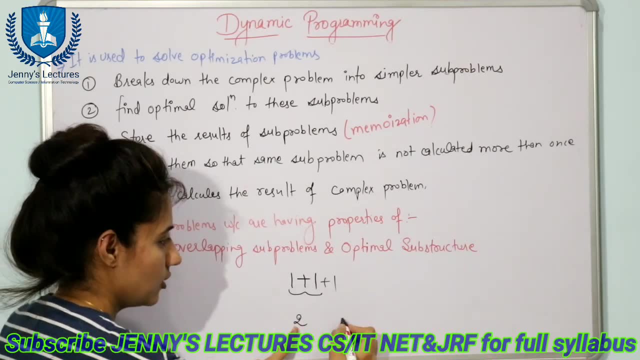 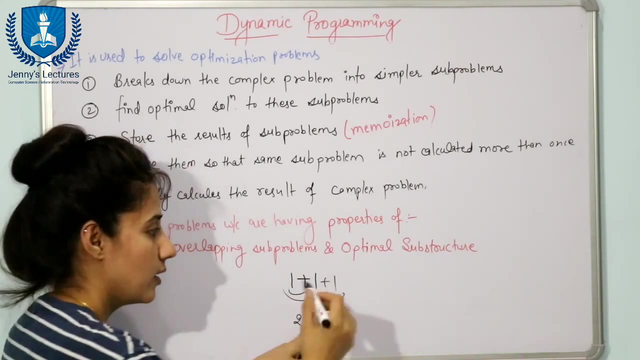 is 2, and suppose this result we store somewhere. and if suppose I add one more, 1, then simply you can say 2 plus 1, that is it. it would be 3, right, and we also store store the result of this one. again, if i add one, then simply you can say three. see, this one is. 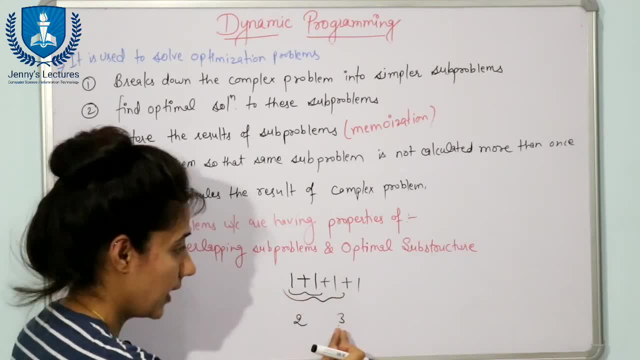 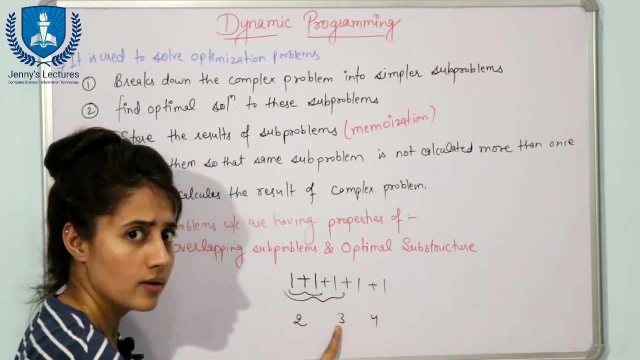 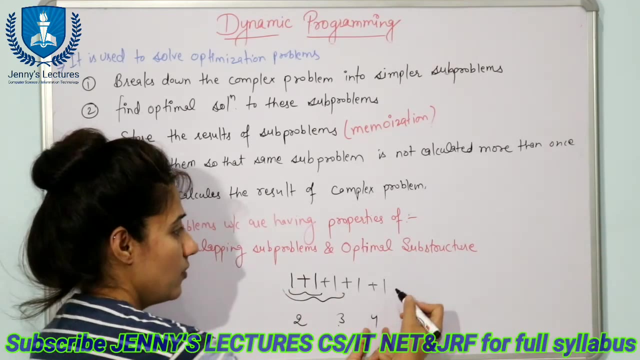 the result of this one. we know because we have stored that result. that is three. so simply add one to this three, that would be four. fine, if again i add one, then i have the result of this sub problem, because i have stored the result of this one. if i add plus one, then i can say this: 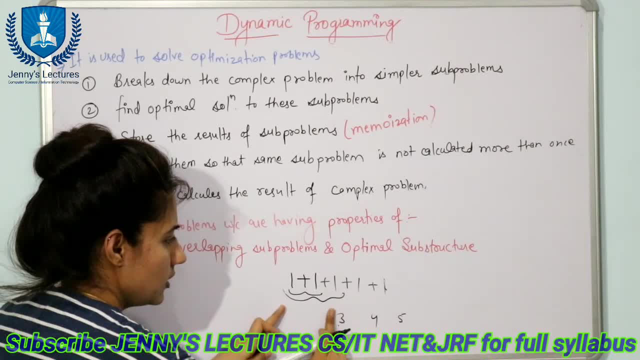 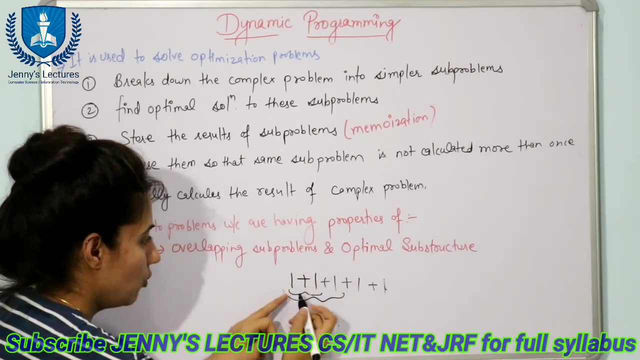 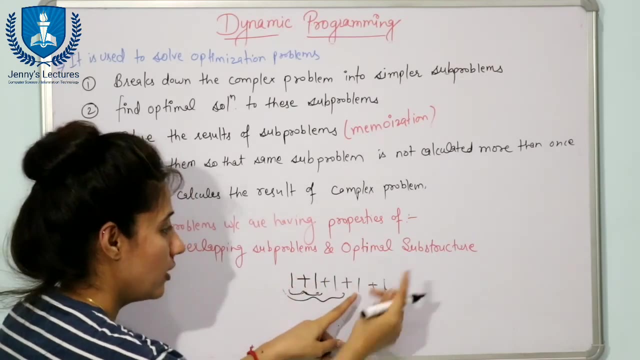 would be five. so if you don't store these results then you have to recompute again and again. see, one plus one is two. now again, if i add one, then i- i don't know this, i don't know the result of the sub problem, so i have to compute: one plus one plus one, that is three. again, if i'm adding one, then you: 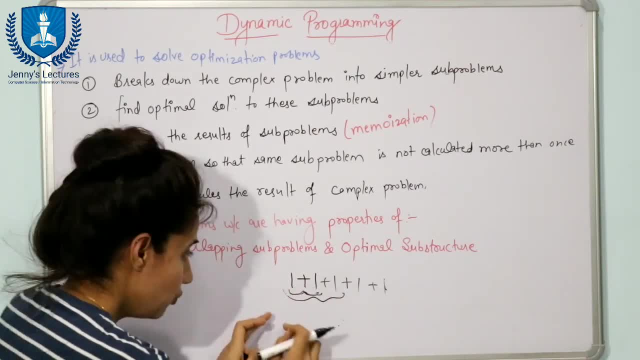 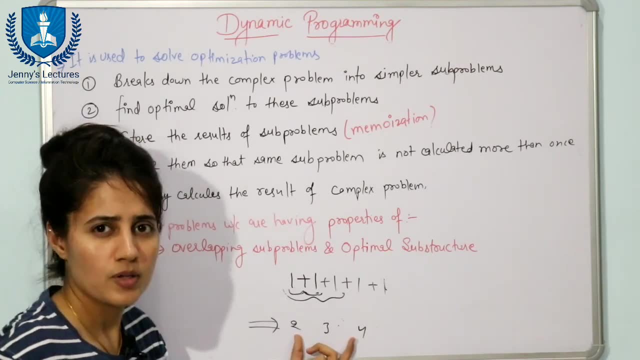 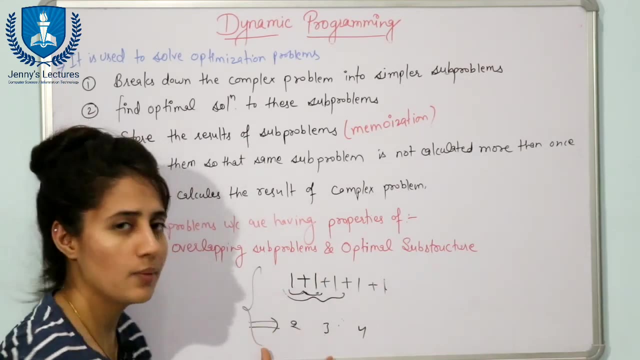 have to recompute one plus one plus one plus one, that is four. if you do not store the values- two, three, four, something like this, fine. so when you store these values, then obviously the calculation or the calculation or the computation of complex problem would be easy, right? so this is what the basics of dynamic 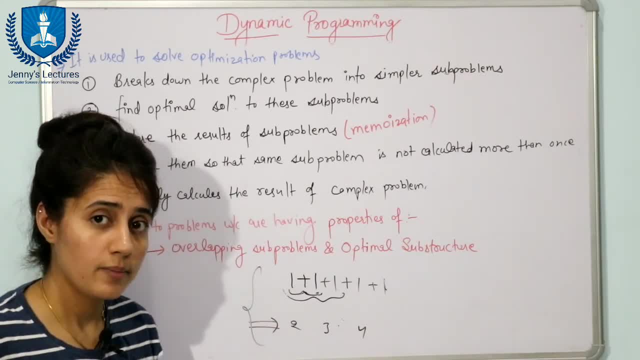 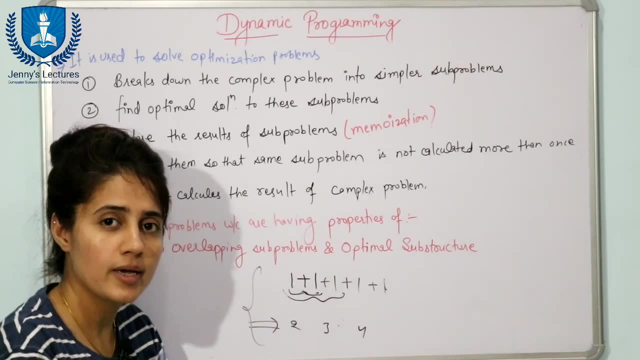 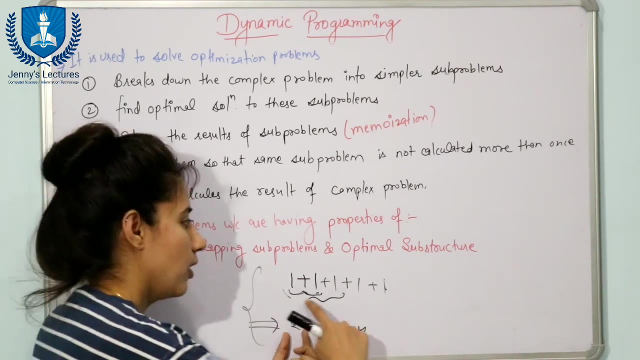 programming. so see, that is the advantage of dynamic programming. so if you store these results, then you don't have to recompute that same sub problem again and again. fine, you just check the result. fine, and you can. you can use that stored result to find out the solution of. 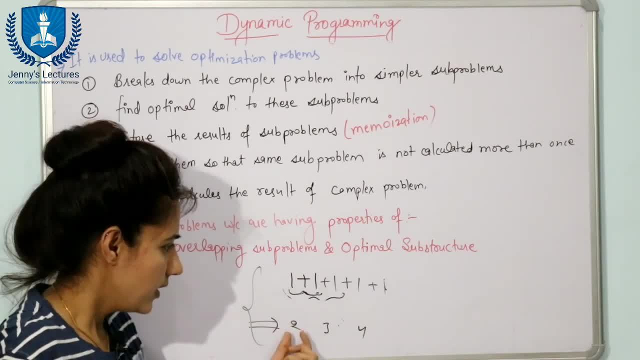 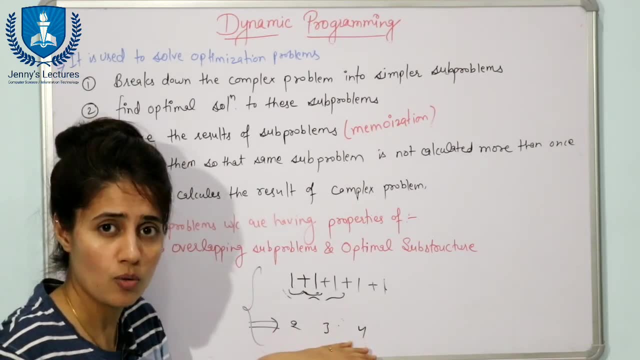 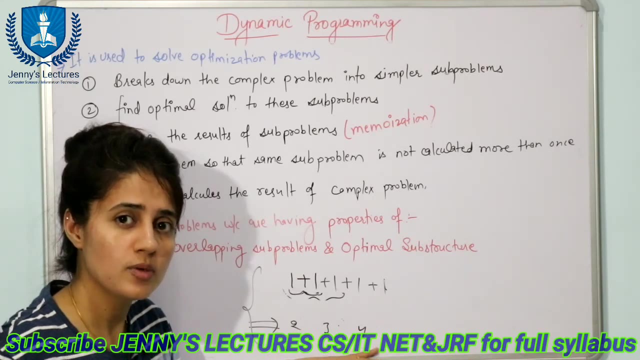 to find out the solution of a complex problem. so it it you can say time complexity would be less. obviously space would be. it would increase the space complexity because you are storing the intermediate results also, so to somewhat space complexity would be increased, but time complexity would. time complexity would be decreased. now i am going to discuss this. 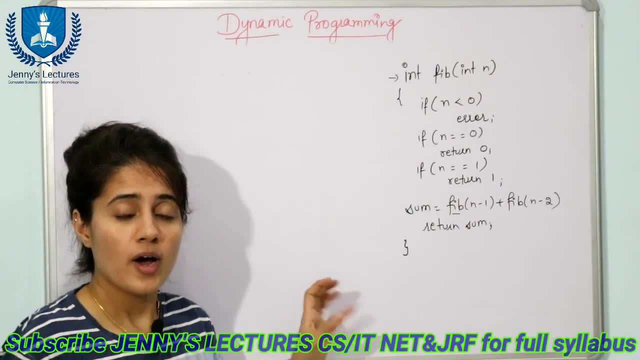 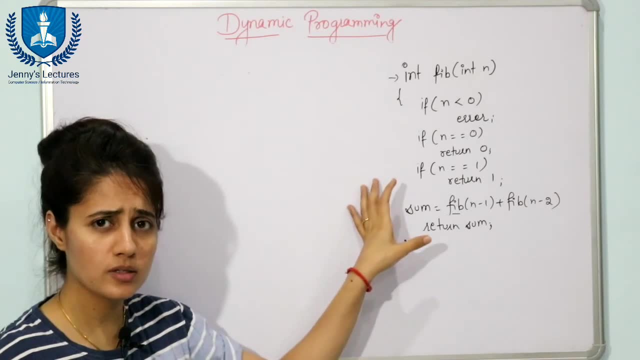 funda with the help of an example. so now we are going to see why we use dynamic program. but you can say what are the benefits of using dynamic programming approach. let us take one simple example. we are going to take the example of dynamic programming. we are going to use dynamic programming. 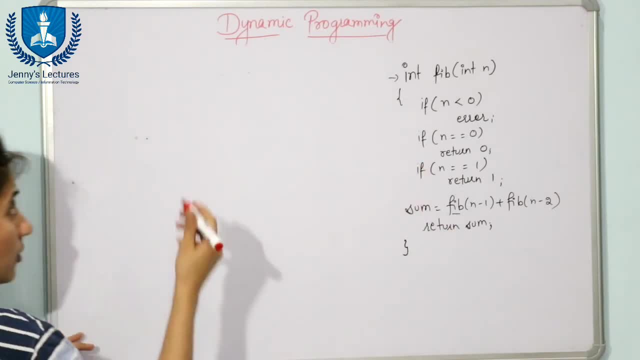 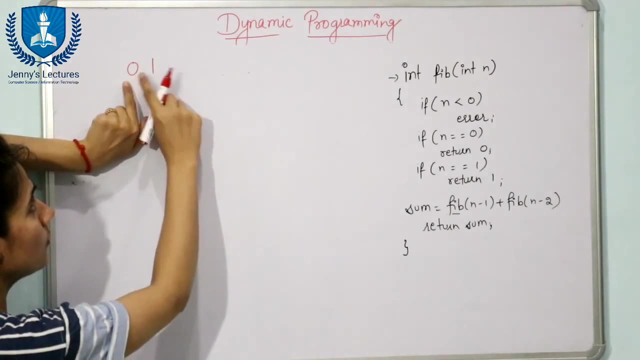 as an example of the febernike series. fine, i hope everybody knows what is the beneses series. first number would be zero and one next number would be calculated by i adding the previous two numbers. one plus zero is one, this number would be calculated. one plus one is two: this number would be calculated. 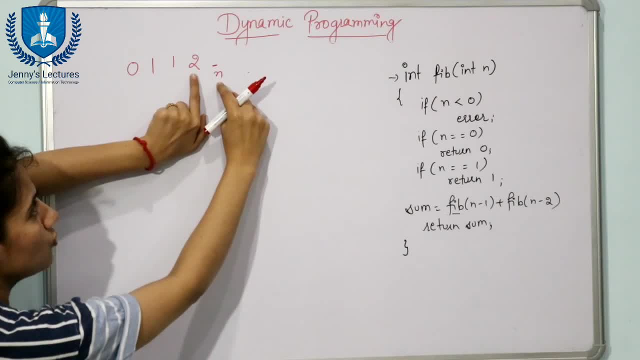 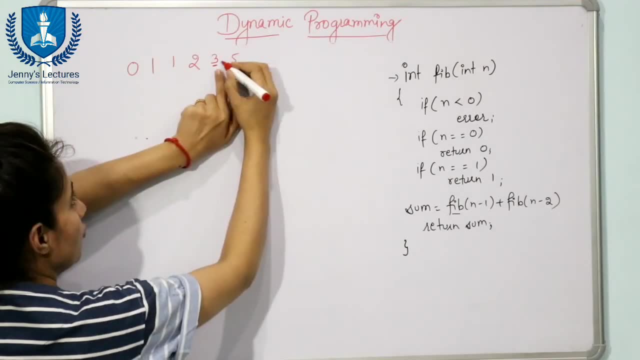 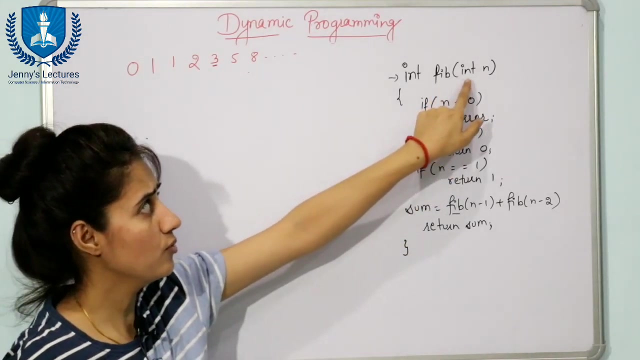 see. suppose this one is nth number, then this would be calculated by n minus one plus n minus two. these two numbers, two plus one is three, then five plus three is eight, five plus three is eight, and like this. so this is the method. if number is negative, we are taking one function, feb. we will pass. 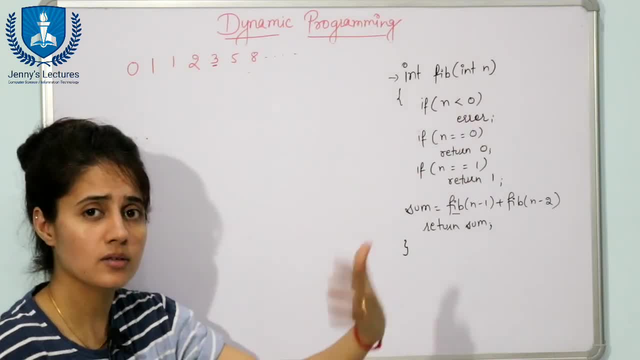 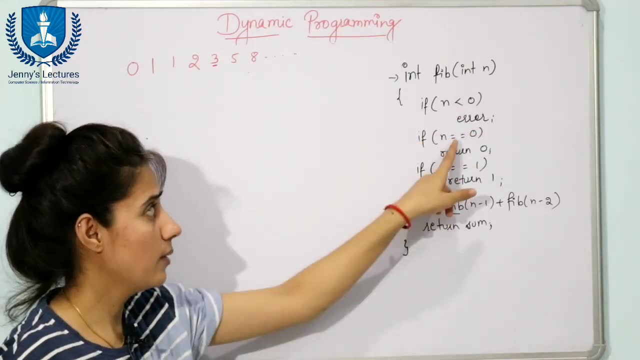 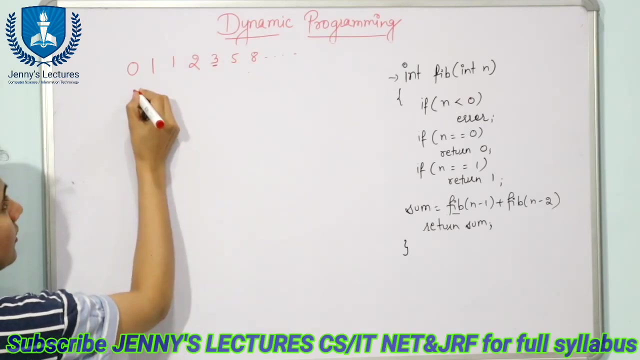 the n value of n because we are finding the nth number of the febuniki series. now, if n is less than 0 means number is negative. then error message would be printed. if number is n is equal to 0, then it will return 0. if n is equal to 1, it will return 1, because see, n value is like something. 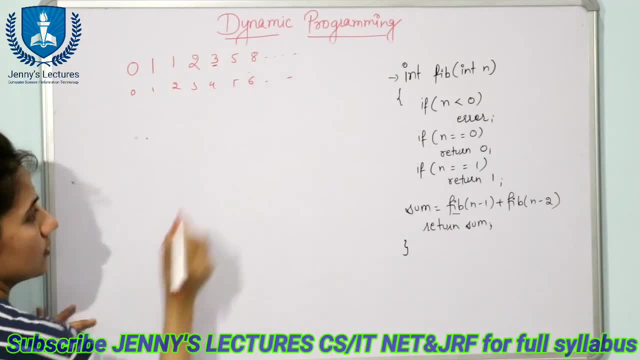 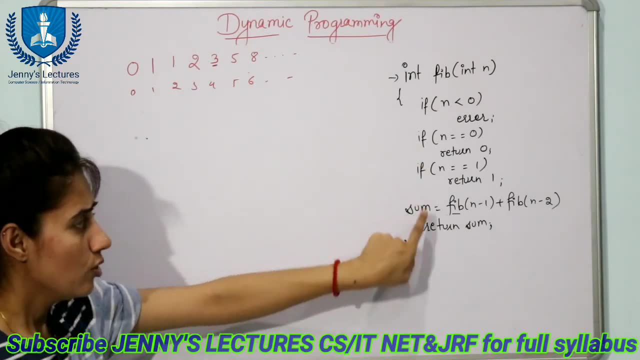 like this: 0, 1, 2, 3, 4, 5, 6 and like this. so if n value is 0, then value is 0. if n value is 1, then value is 1. if this condition is not true, then what will happen? next value would be calculated by n. 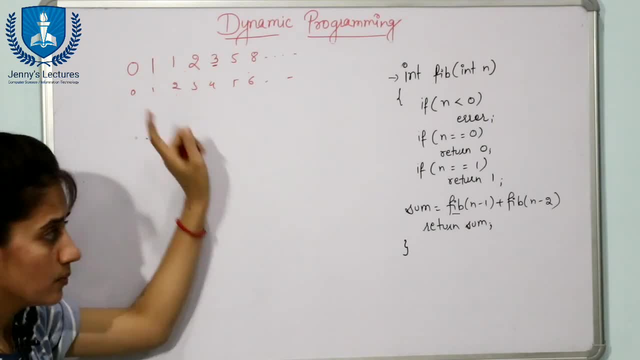 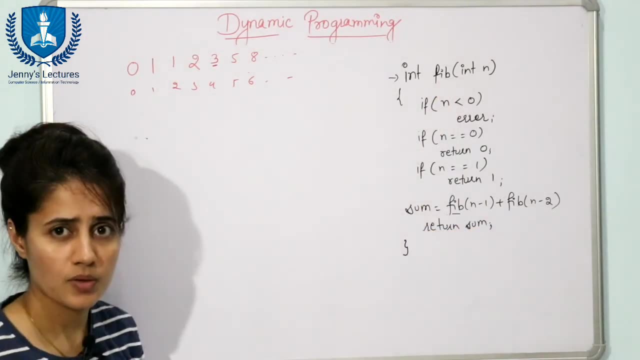 plus 1, n plus sorry, n minus 1 plus n minus 2. so again we will call, we will call this function feb of n minus 1 plus feb of n minus 2, and then we will return this sum. so now, i hope you can. 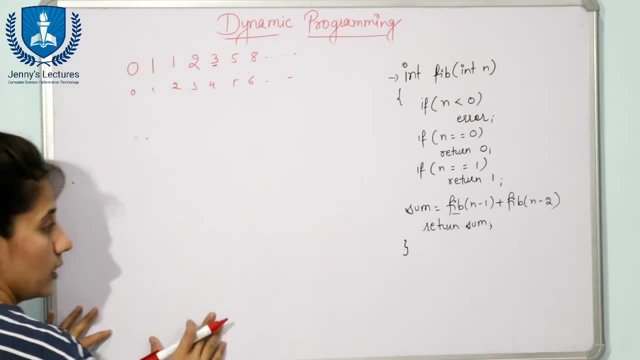 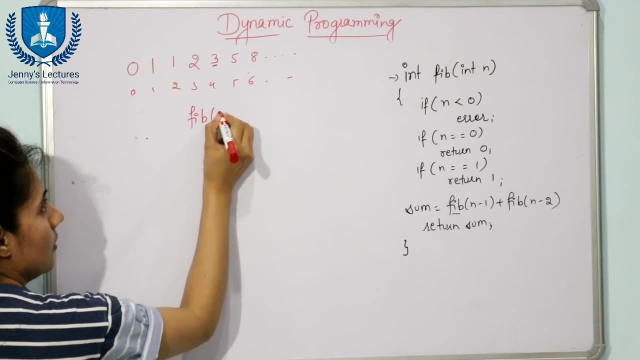 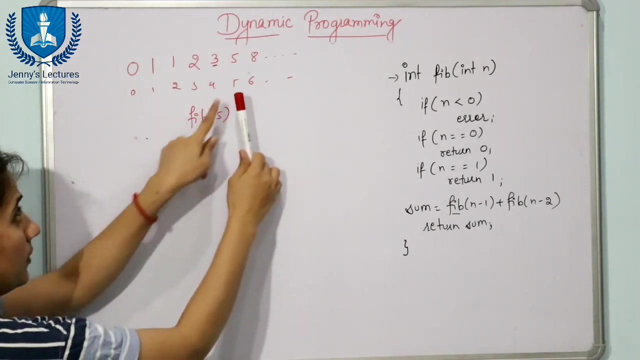 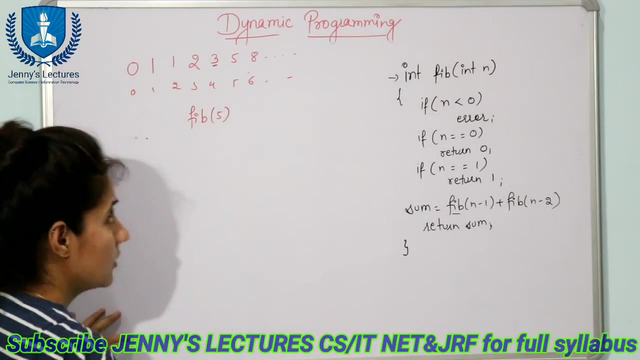 easily write down the code for this feb. how to print this febuniki number. fine, now see if we are taking the value 5, if we are passing the n value is equal to 5. we are calculating the fifth number means fifth number would be 5. then 5 would be printed. then what is the flow of execution according to this code? see: 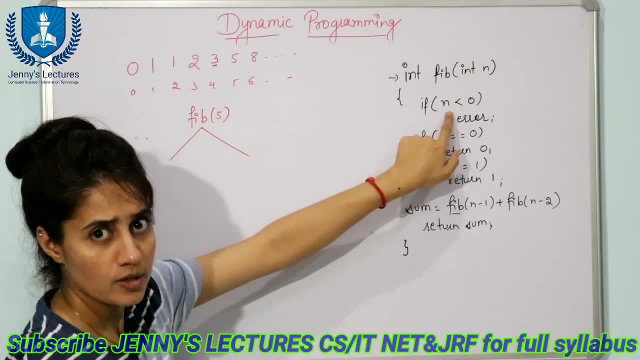 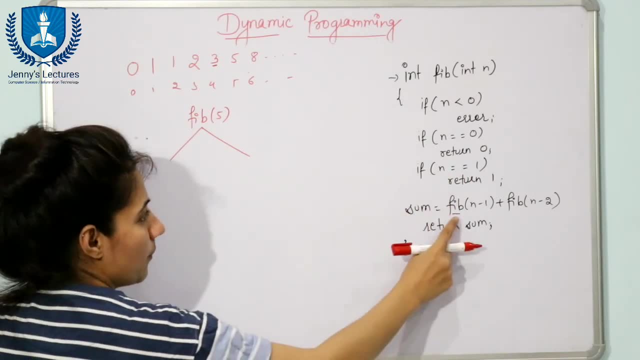 here we have. this condition is not true because 5 is not less than 0. this condition is not true. this condition is not true, then, finally, control will go to this line. now what will happen? sum is equal to feb of. again, the same function would be called: 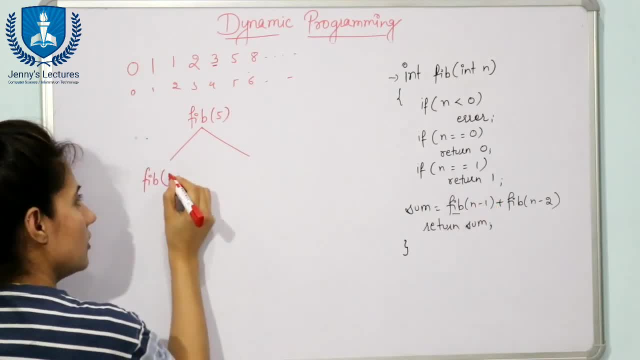 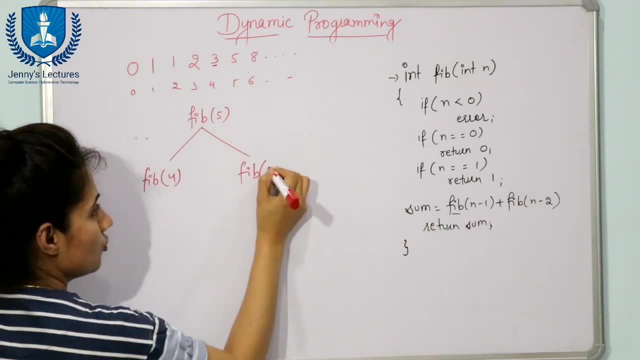 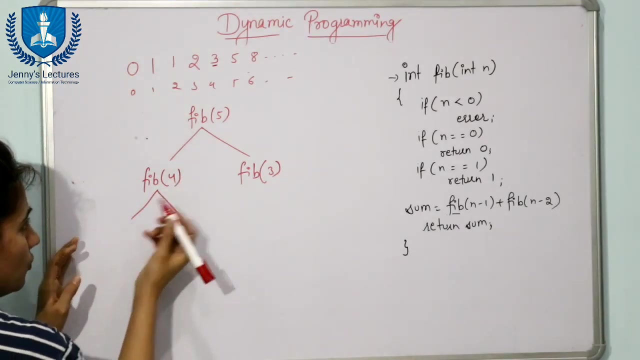 n minus 1. n is what? 5, 5 minus 1, that is 4 plus plus. here what will happen? the second is n minus 2, that is 5 minus 2 is 3. fine, next control would go first of all. this side would be executed. 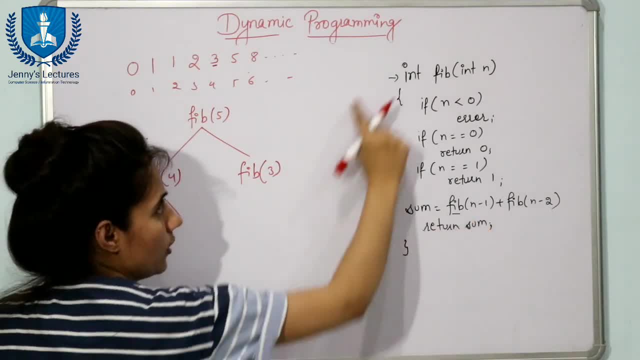 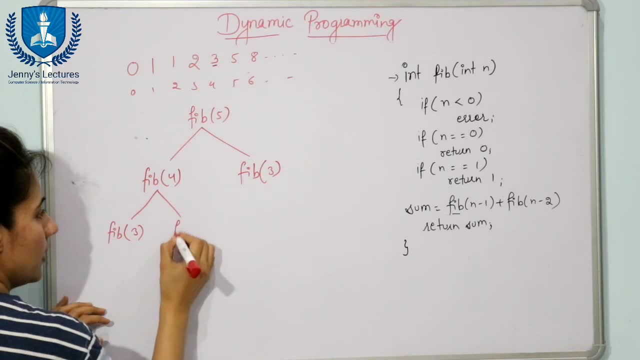 now here: if 4 is again, this 4 value is to be passed. this is not true. this condition is not true. this condition is not true. then again, feb is called 4 minus 1, that is 3, and here what we will have: feb of 2, again feb of 2 and feb of 1, again feb of 1 and feb of 0. fine, now we cannot. 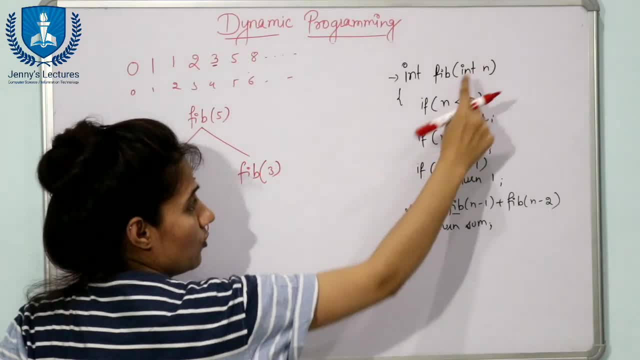 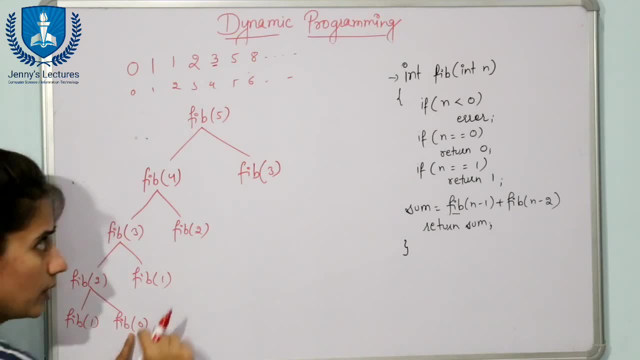 expand this one because when 1 is to be passed, then what will happen? this condition is true, so it will return what 1. fine, So we are not going to expand this one. when 0 is to be passed, then it will return what 0. ok, now see this side. now see this: feb of 2, feb of 1 and feb of 0. now, after completing, 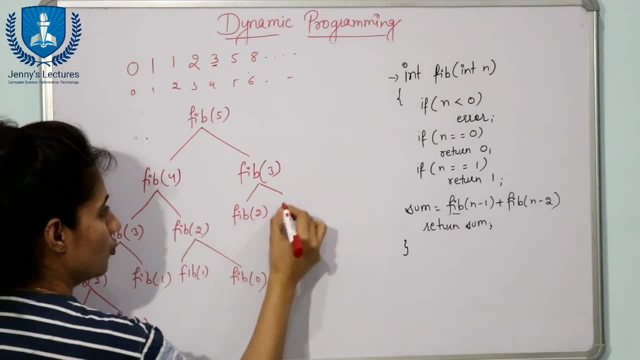 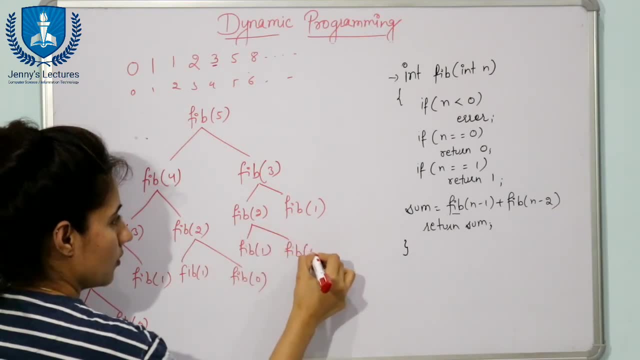 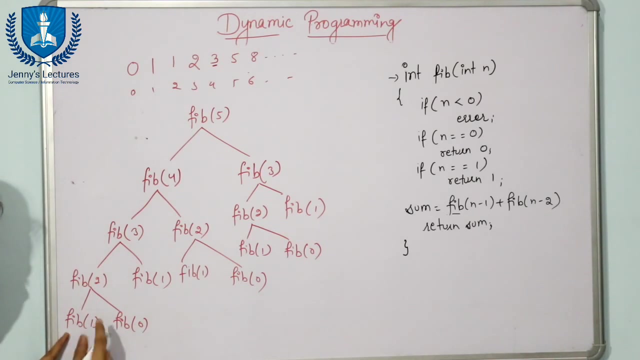 this side. this will be feb of 2 and 1. this would be feb of 1- 0. so this would be the recursion transition. Now how the values to be calculated: see this: feb of 1. it will return what 1 and it will. 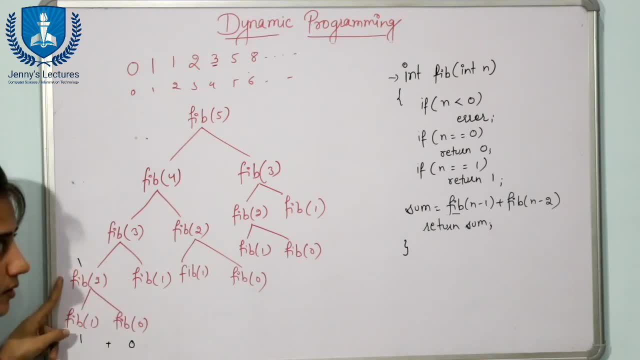 return what 0. 1 plus 0. it is what 1, because we are going to add these numbers. fine, now this 1 plus feb of 1. this will return what 1. 1 plus 1 is what 2. now this side feb of 2. but here we. 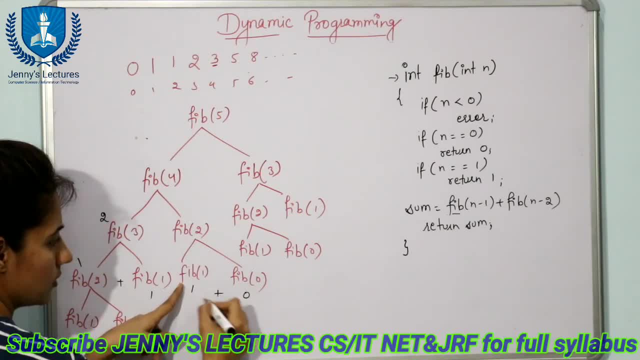 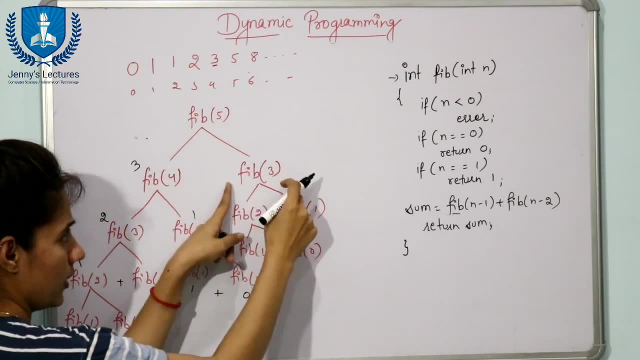 have feb of 1, feb of 0. this will return 1. this will return 0. 1 plus 0 it is what 1. 2 plus 1 is what 3.. Now we can, when we cannot calculate this one, because we are going to calculate first of all. 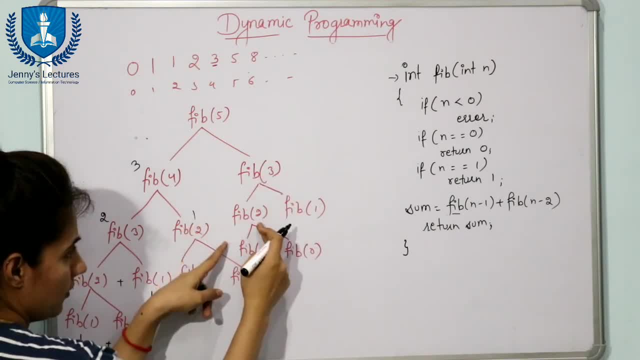 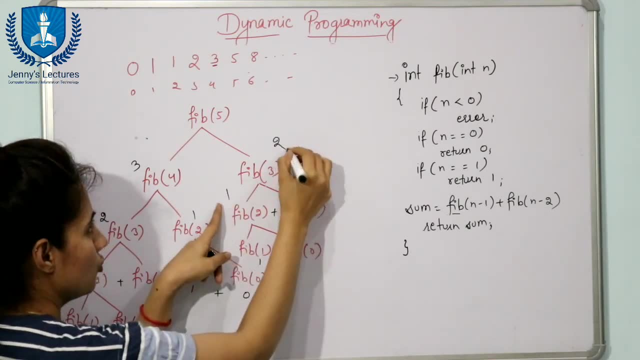 this part: feb of 3, then control. go to this side, left side- then feb of 1 and feb of 0. this will return 1 plus 0, that is 1. this will return 1. 1 plus 1 is 2, 3 plus 2 is what 5 and the value will. 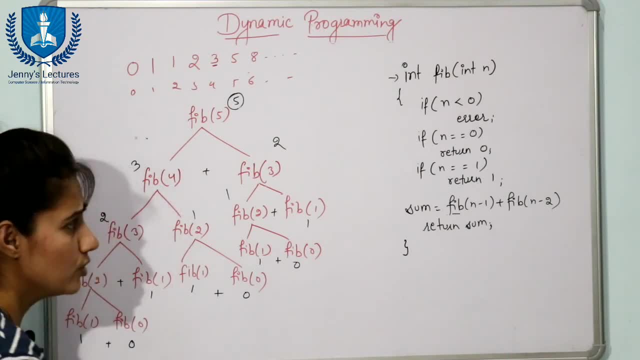 be printed as 5. fine, so this is. this is the you know, recursive method. now what is the drawback of using this recursion? see In the execution. it is going to solve this part first, feb of 4, then feb of 3. this, this part first. 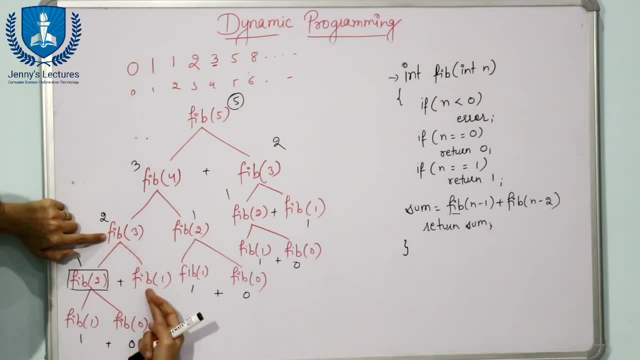 like this one. fine, then, to calculate this one, we need this one. then this would be solved and the answer would be 2. then, for solving this one, this would be solved, this would be solved, and again, 2 plus 1 is 3. now this is something known as overlapping sub problems. why? because, see we, 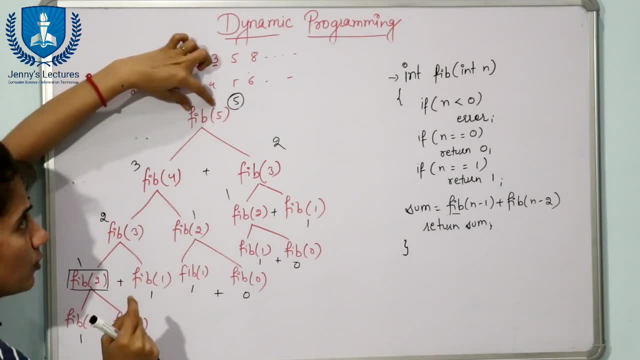 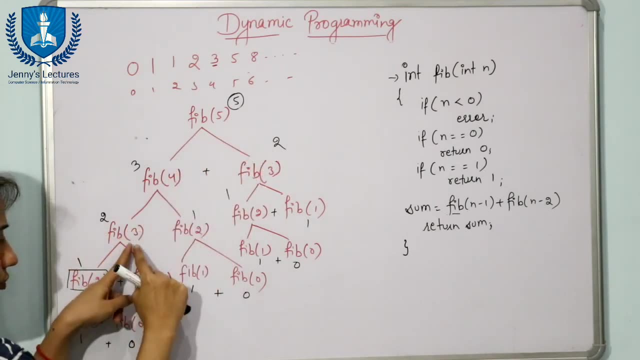 are calculating the any number. we are calculating febuniki series for number 5. so we have divided this problem into sub problems, see for 4, for 3, we are calculating. for 2, we are calculating. so these are sub problems. now and these sub problems are, we are using these sub problems again and 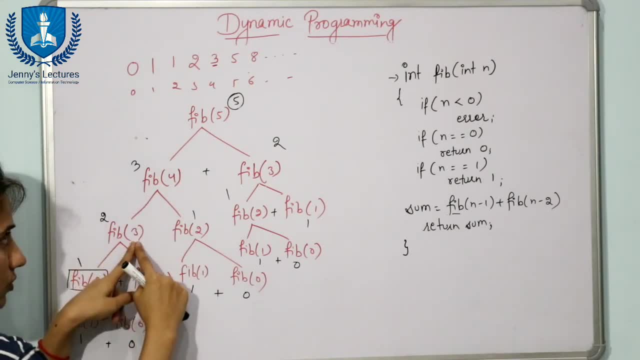 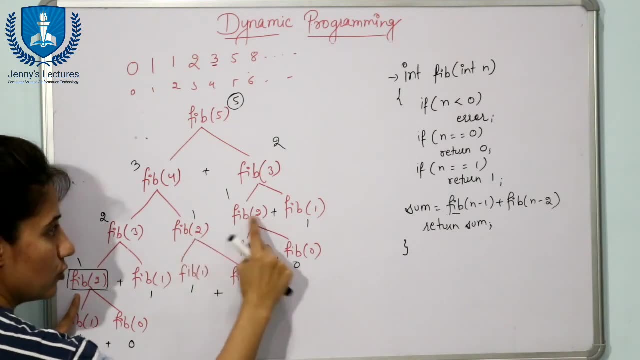 again more than one time. see this: feb 3 is here. we are using feb 3. here also we are calculating for febuniki 3. here we are calculating for febuniki 2. here also we are calculating for 2, here also we. 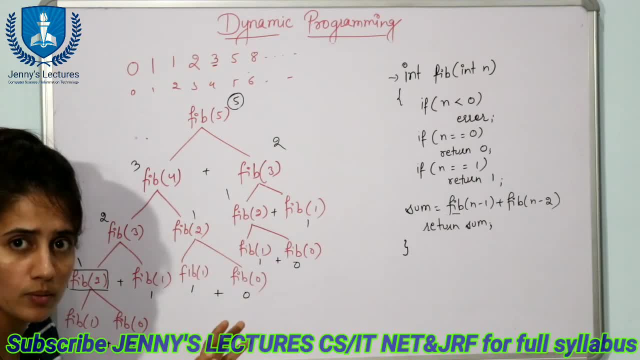 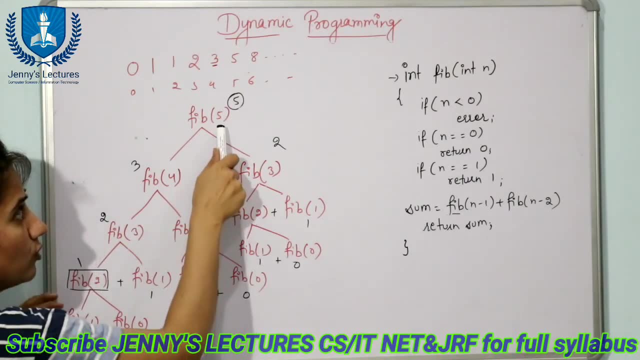 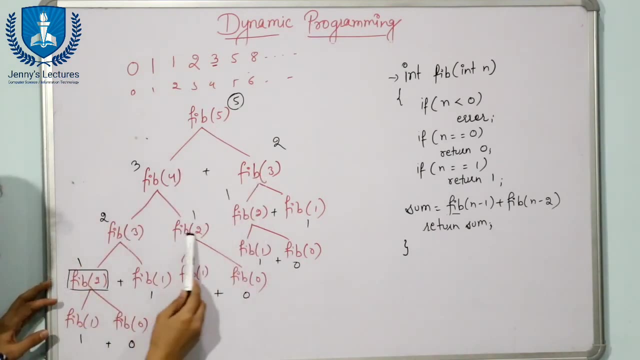 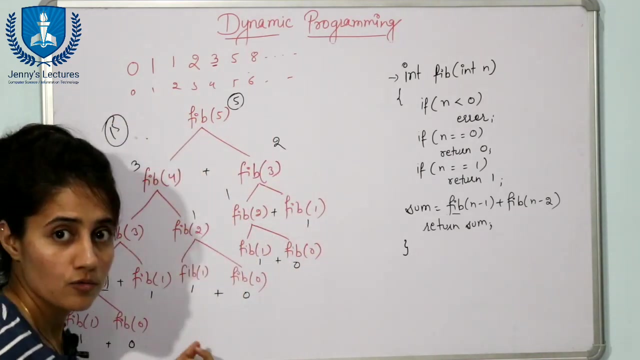 are calculating for 2, so again and again we are using same sub problems, so this is something known as overlapping sub problems. Now, in case of recursion, when n value is 5, then how many times this feb function has been called? it is almost 1, 2, 3, 4, 5, 6, 7, 8, 9, 10, 11, 12, 13, 14, 15, 15 times, 15 times this febuniki function would. 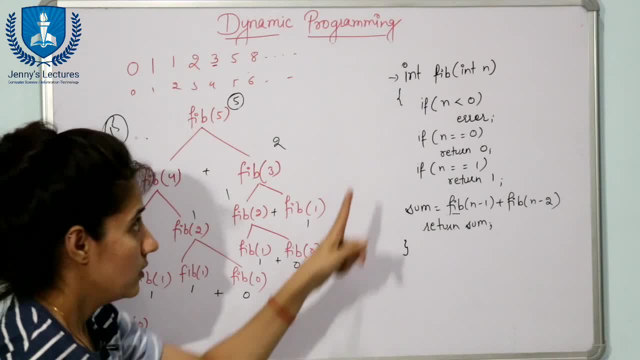 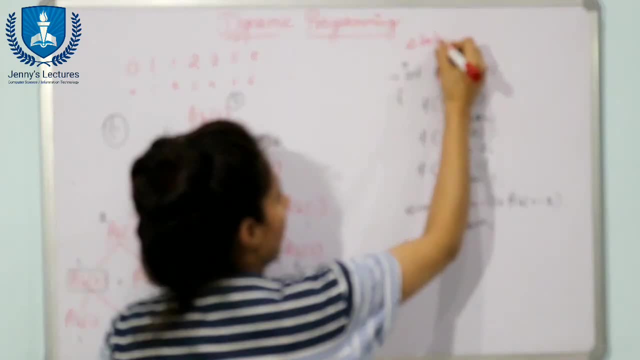 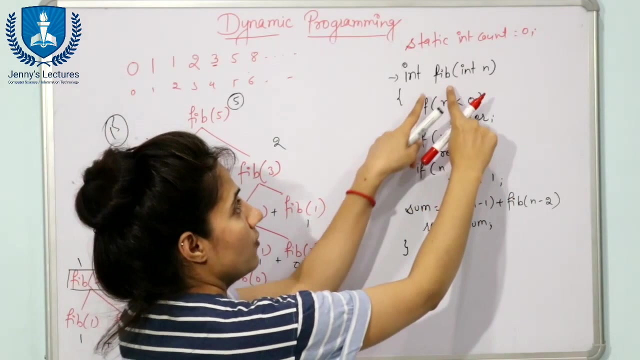 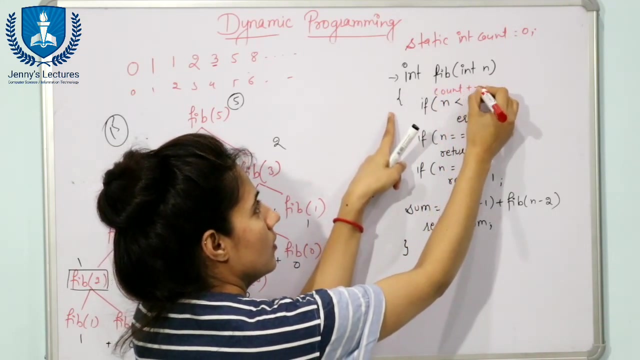 be called, and if you want to calculate this count value, then you just have to modify this code something like this: you just take a count variable, static int. count is equal to 0, and after you know, in the definition of this function, after this bracket, you just write count plus plus, fine, and when you are printing this sum in the main, 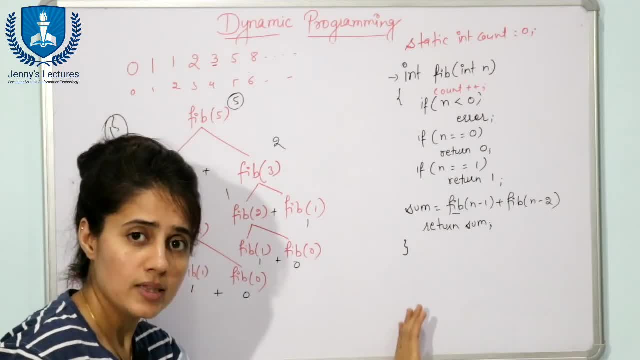 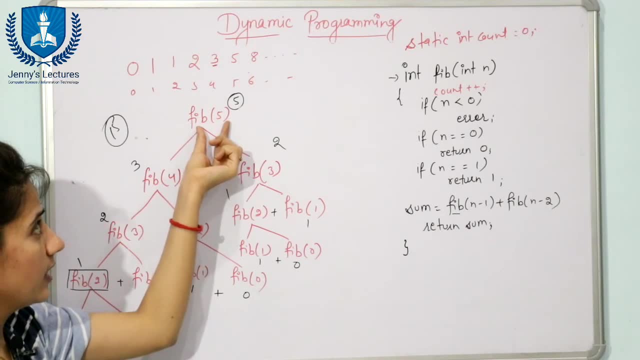 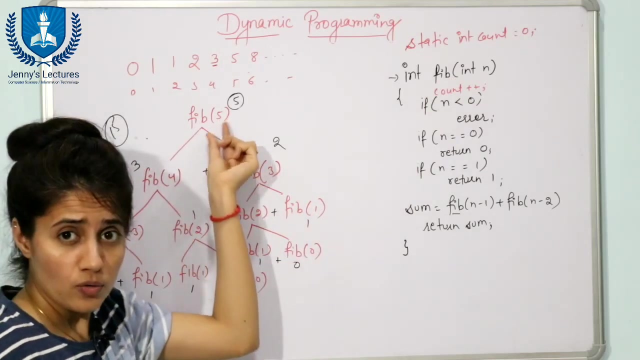 function. obviously you will write some main function. then in that main function you can print this count and then you will get to know that when you will pass n is equal to 5, then this 15 calls would be made to this function. so when this n, when you will. 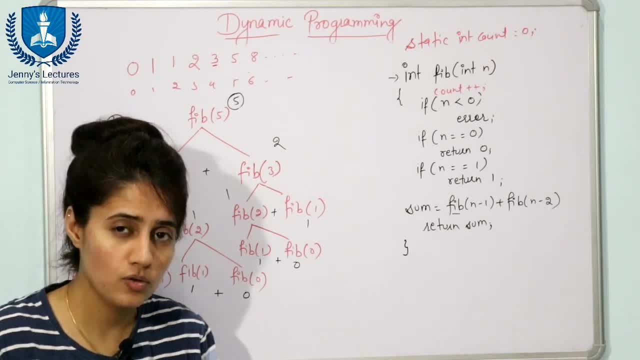 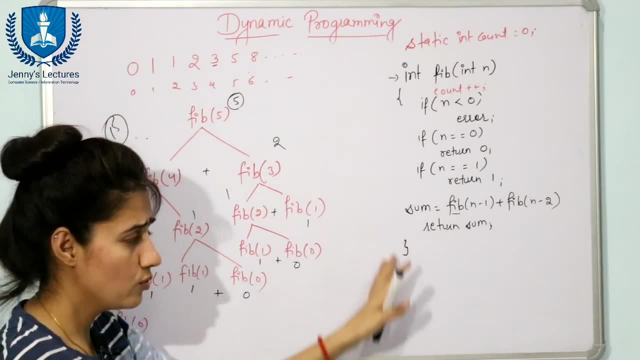 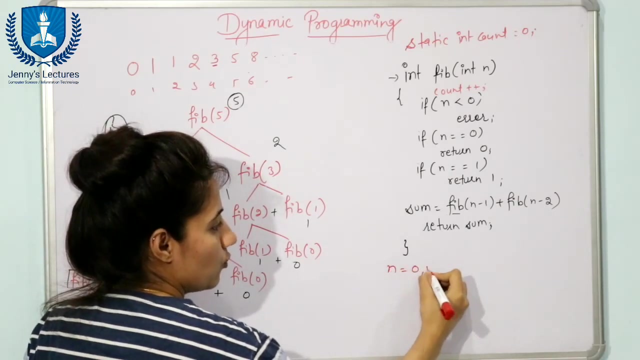 increase this n value, then you will notice that you will have to wait for some time to get the output. why so? because of the computations. you just write down the score and try to print this count number. see something like this: when n value is 0 and 1, then count would be 1 only. so see when: 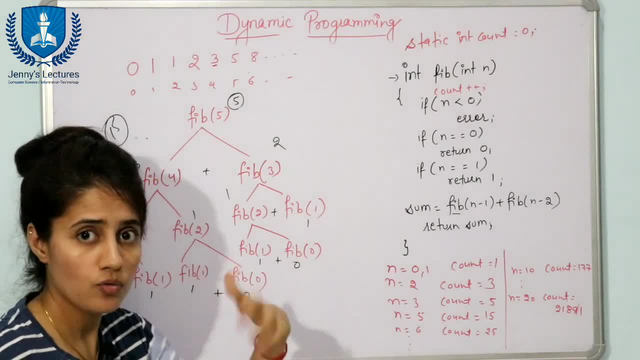 you increase this n value, then you will get to know that when you will pass this n value, then you will get to know that when you will pass this n value, then number of function call would be increased and then the number of the computation time would increase and obviously the time complexity. 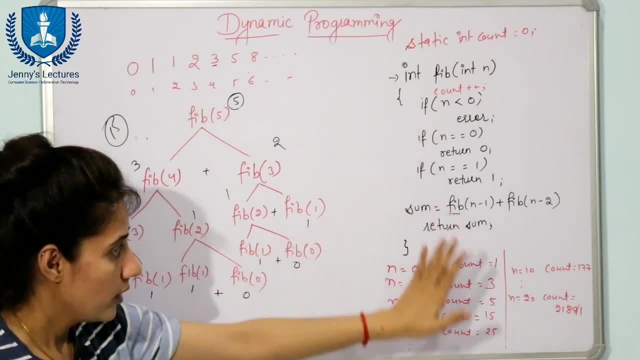 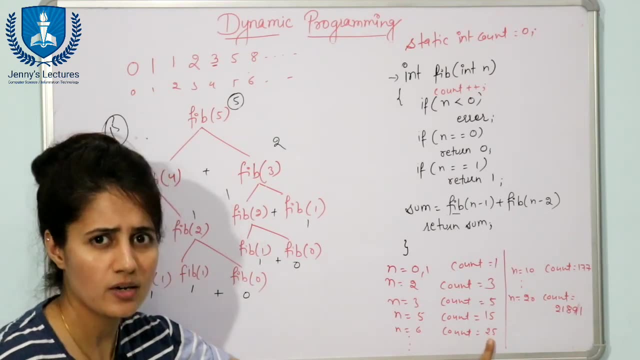 would also increase. now, if you write down this code and try to execute this code, then for n is equal to 2, 3, 5, 6, the count would be up to 25. that is fine. but when n is equal to 10, then count would. 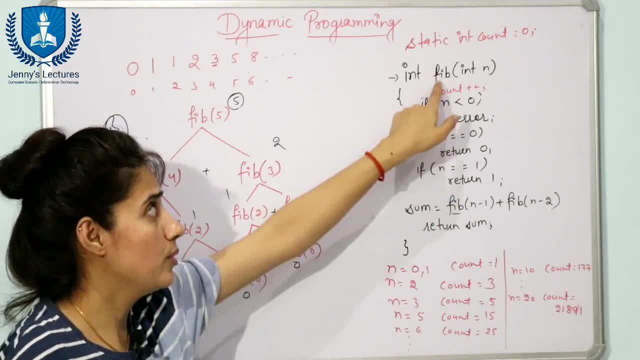 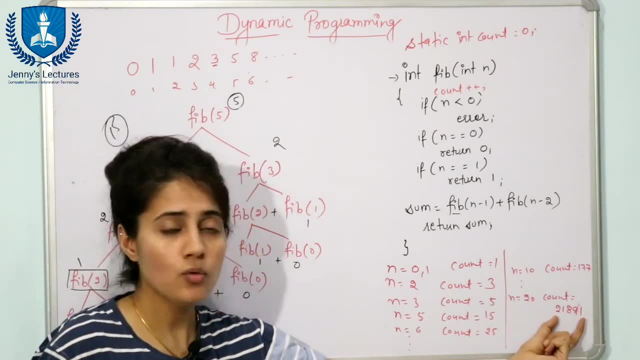 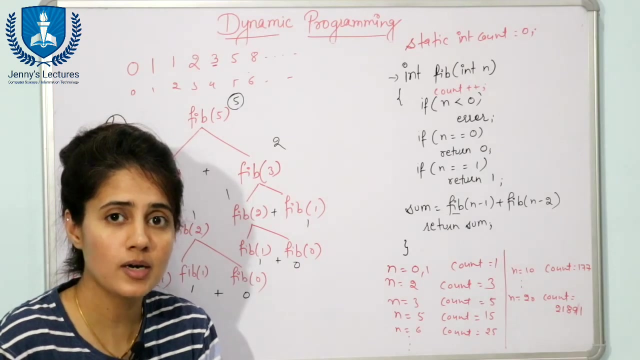 be 177, 177 times. this fibonacci function would be called just for value 10.. when n is equal to 20, then count would be 21 around 20, 2000. so see, this would be increasing exponentially. you can see approximately exponentially. so when you are using this recursion type of 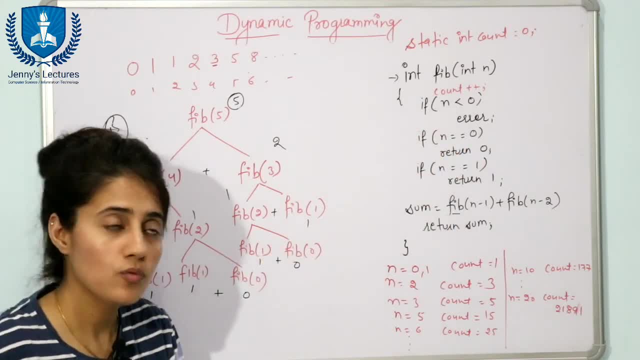 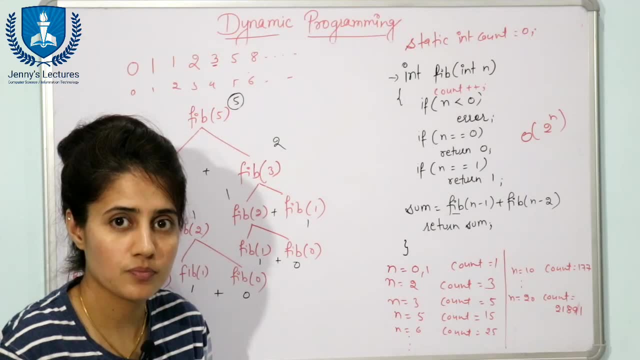 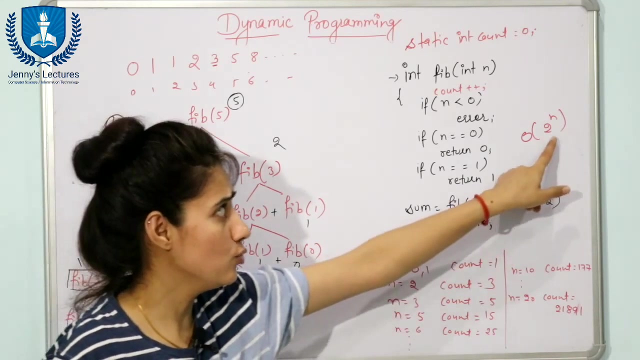 method to solve this problem. then the time complexity would be: what order of 2 raise to power n? it is taking exponential time. when you are increasing this n value, then count value is increasing exponential. you can say 2 raise to power n. so see when, see as you see exponentially when n is. 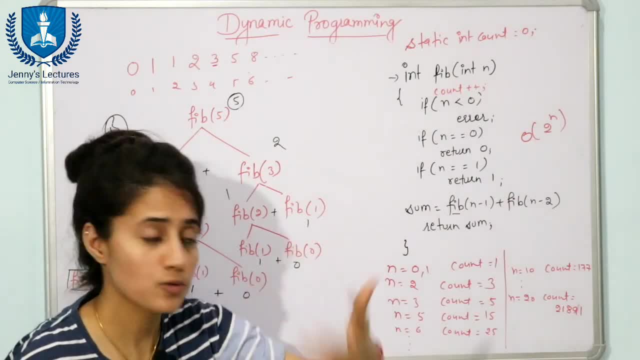 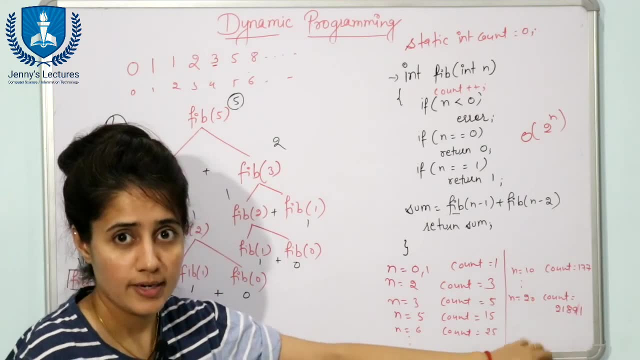 equal to 20. then how many times this fib function has been called? around 22000 times. approximately 2 raise to power n. you can say approximately 2 raise to power 20. it is not exactly 2 raise to power 20, but then when the n values would be increased then it would be approximately 2 raise. 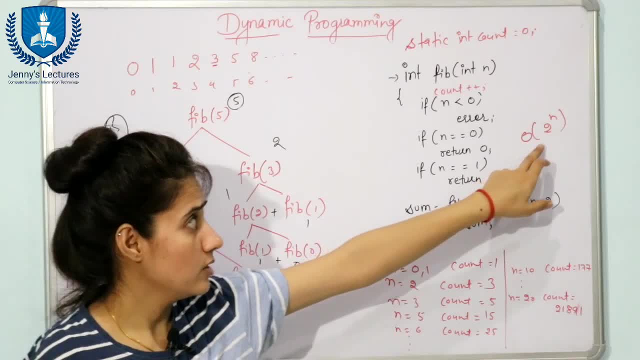 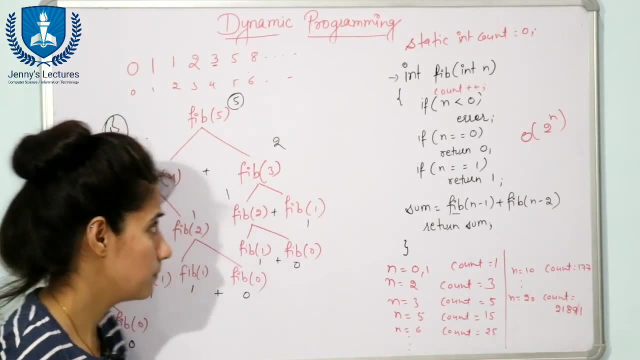 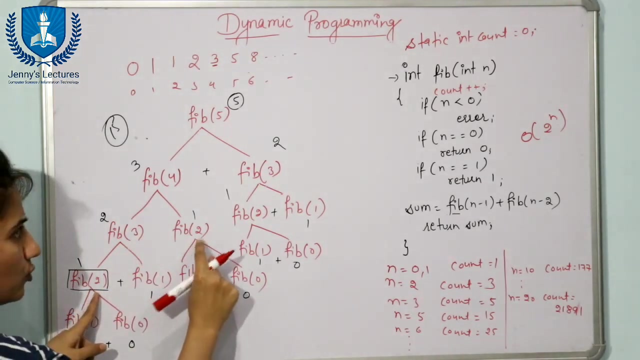 to power n. fine, so that this is this time. complexity is very high. and why so? why so? see here this. this fib 2 is here. we are calling this fib 2 again, fib 2, again, fib 2. every time when the same function is the same sub problem is called the recursive tree, for this problem has been 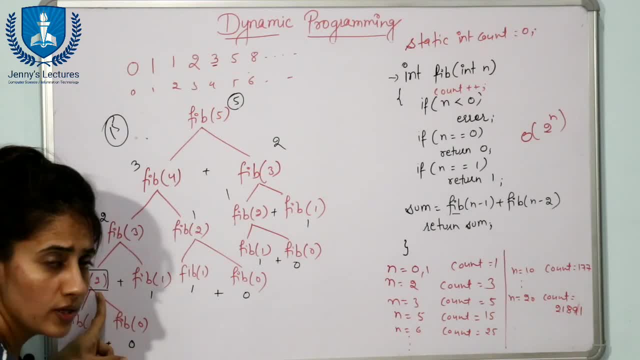 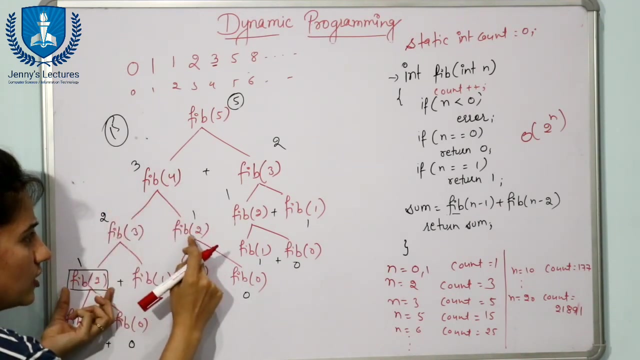 generated. So one solution is: rather than generating again and again this recursive sub tree, can't we use the previous calculated value? because once we have calculated this value now, now again, when, when we will say this, fib 2, then we will not generate this recursive tree, we will just take. 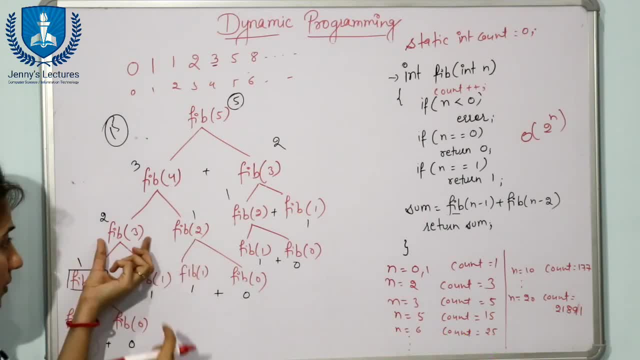 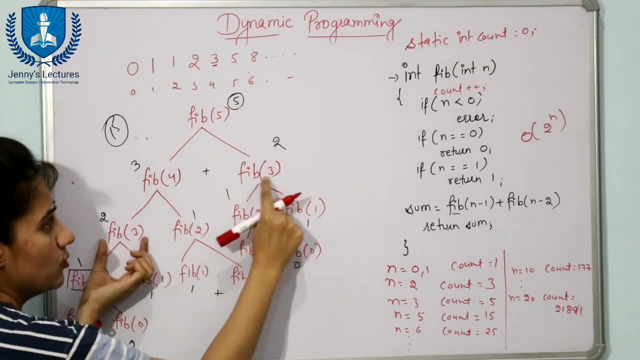 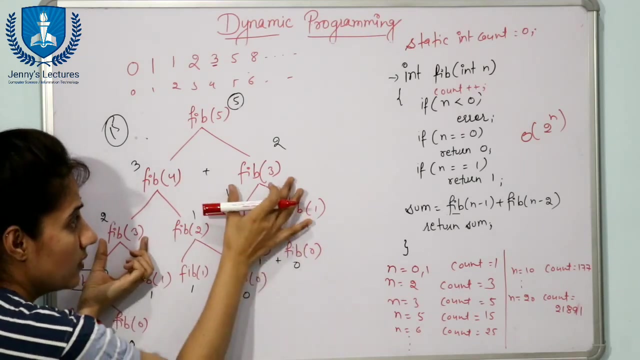 this value. fine, see same with f. fib of 3. we have calculated this value. fib of 3 is equal to 2. now, at this side, when again fib 3 has been called, then if you do not store this value, which happens in this case in recursion case, then again for fib 3, this, this recursive tree, would be generated. so these number. 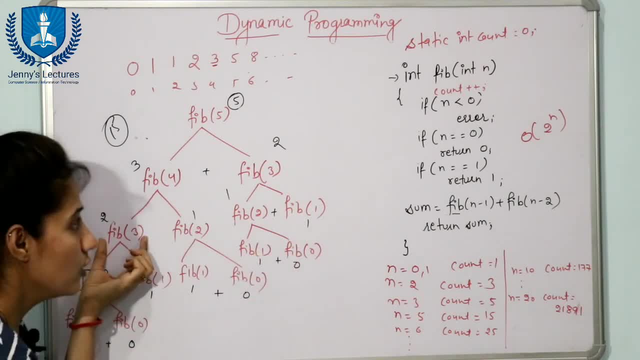 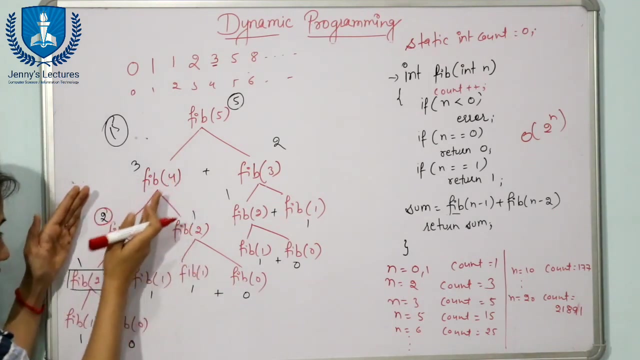 of function call would be there again and again. fine. so rather than calling this fib 3 again, rather than generating the recursive tree for this fib 3, we just can't- we just take this value 2 and use here. and how we can do this? by storing these values. we, just, when we are calculating these values, we just store these. 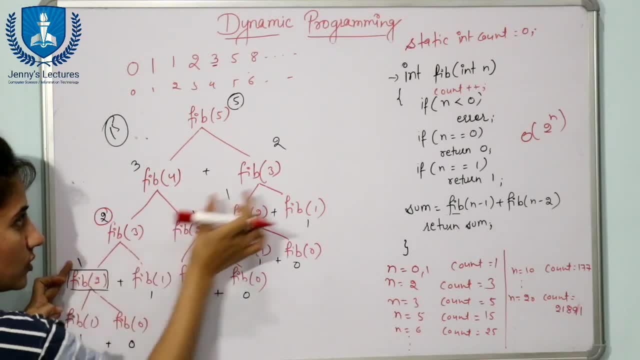 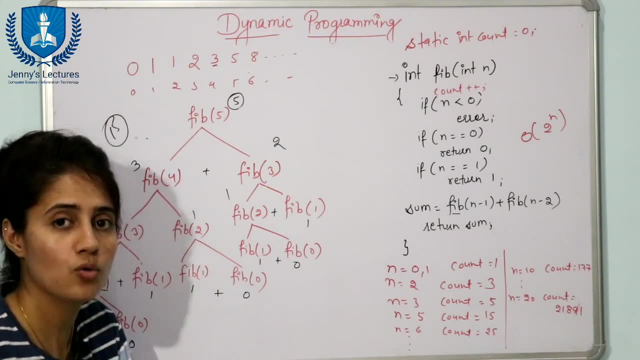 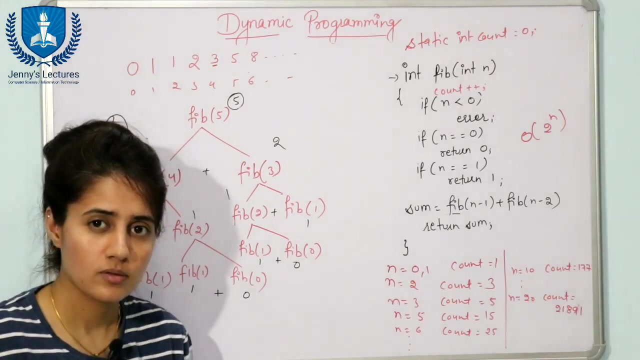 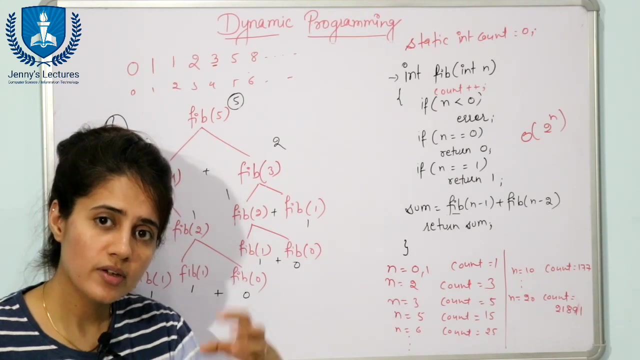 values and again when, when we will see this function, then we just use this value. so this storing of value is known as memoization. now this is basically known as dynamic programming: storing the intermediate result and then reusing those results, so that we don't have to recompute the subproblems again and again. we just recomp, we just compute the. 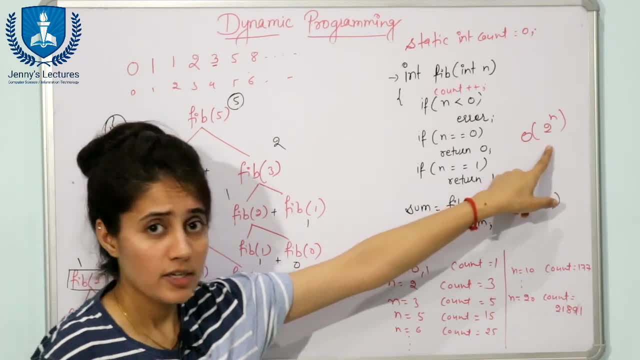 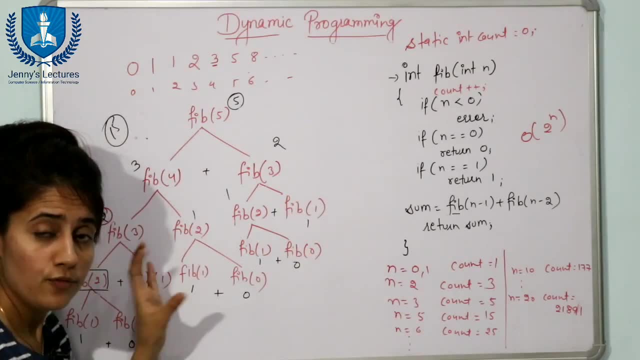 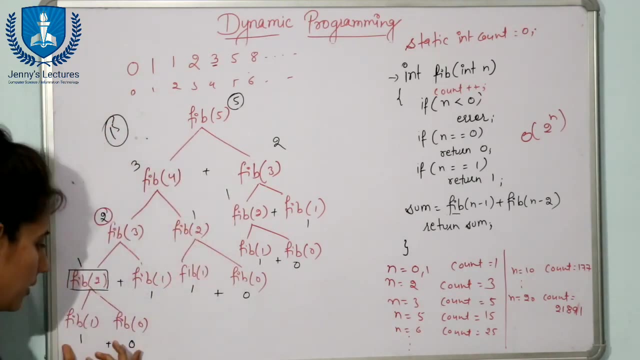 subproblems once, in this case, this time, complexity is why so? because you are recomputing, we are calling that function again and again every time when that function appears. now see, if you, we are applying dynamic programming, then what will happen? obviously, this would be called this recursive tree, would be there now, see. 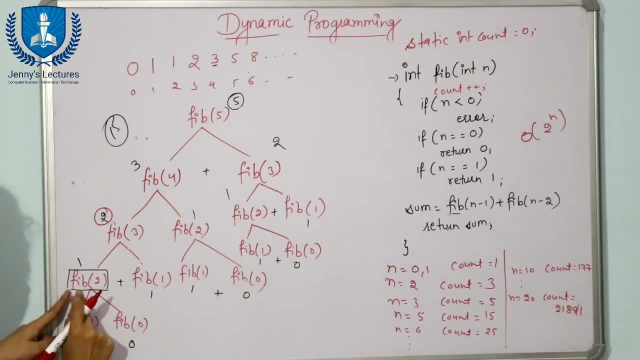 this one is one, this one is zero. we know, okay, when we are, when we find the value of fib 2, then we will store this value. fine, now, when we are going to this fib 2, then we will not call this function fib 1 and we will not code fib 0. why so? because we just take this value and we will use this value. 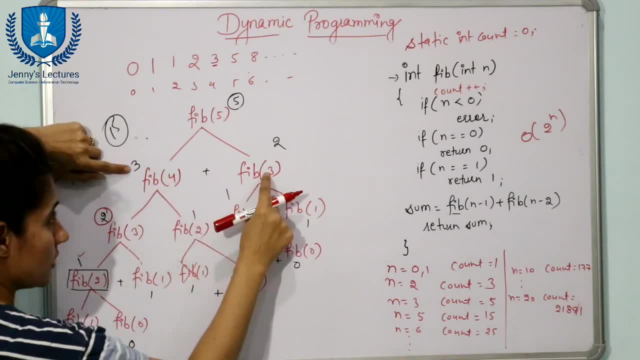 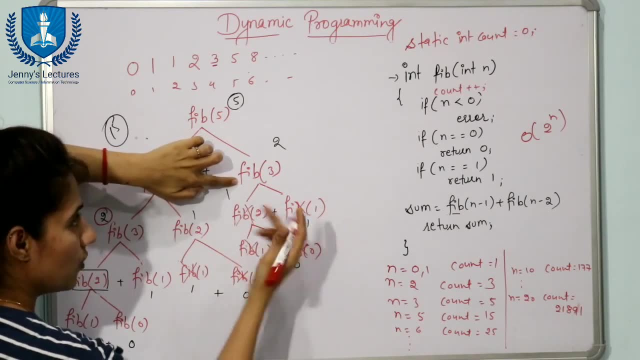 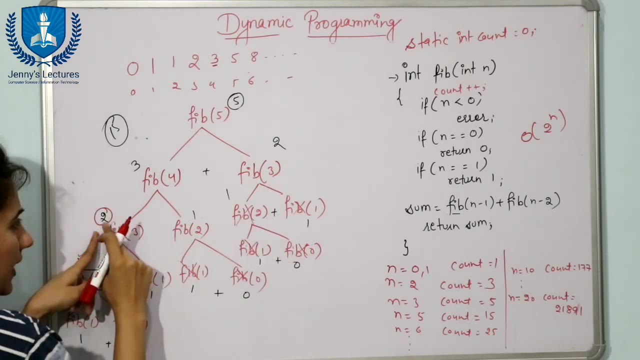 okay, now, 2 plus 1 is 3. now come to this side. when we see this fib 3, we will not call these, we will not generate this tree. why so? because we have, we already have the value of fib 3. we have computed this value and we have stored that value, so we will take just this value 2. so 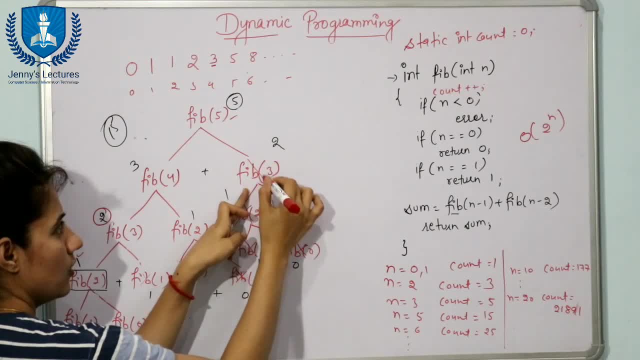 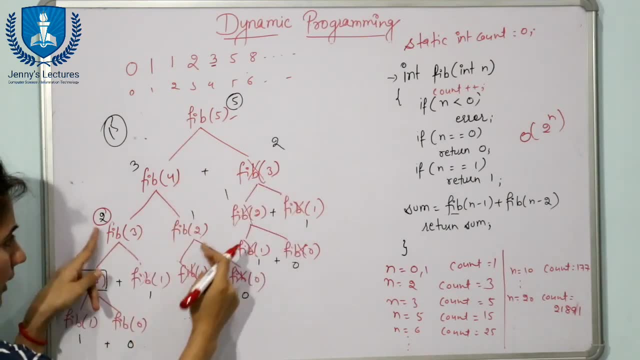 here no need to generate this recursive tree and no need to call this function, also because we are having already the value of fib 3, that is here 2, fine, and here also no need to call this function, fib of 2 and no need to generate this tree, because we have already computed this value. that is. 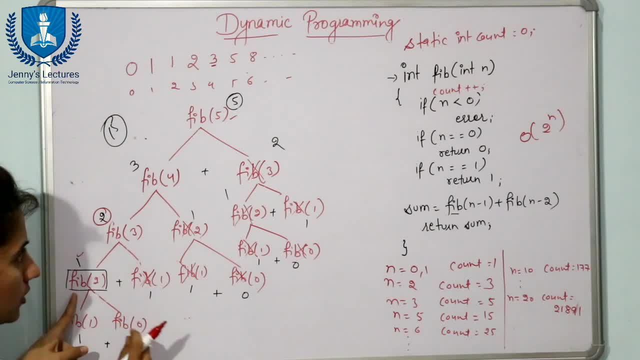 1. here also, we will not call this function. so how many function calls are there in this case? i guess 1, 2, 3, 4, 5 and 6. now n value is 5 and occurs this calls are 6, so obviously that you. 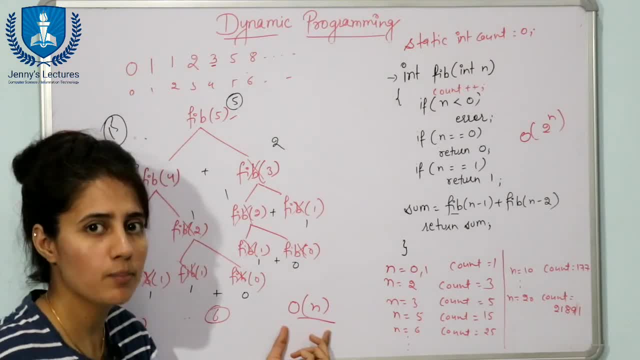 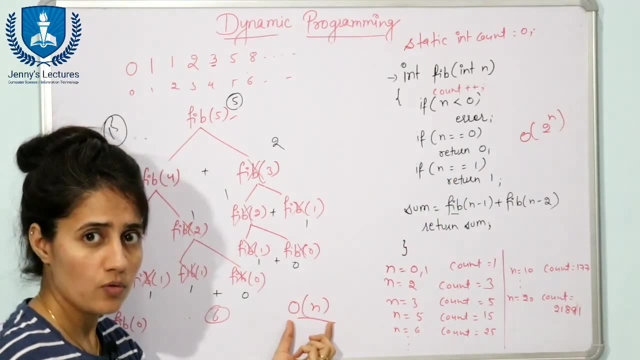 can say the time complexity would be order of n. or you can say n plus 1, that will write order of n. so from 2 raise to power n. we have got time complexity, we have got the time complexity order of n. when you are using this technique, when you are storing the intermediate results, 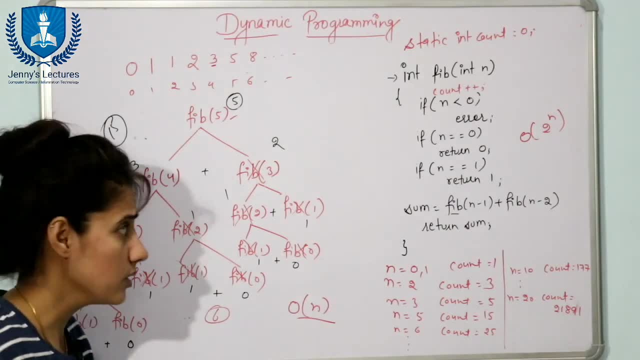 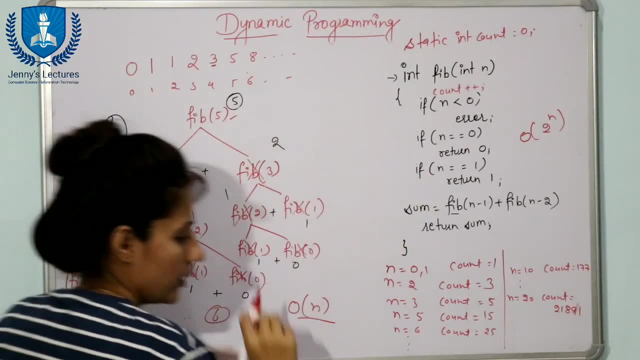 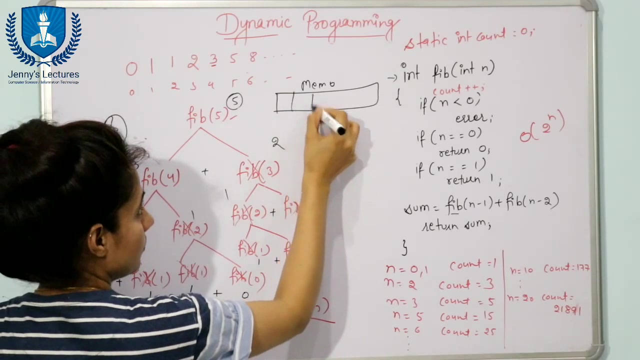 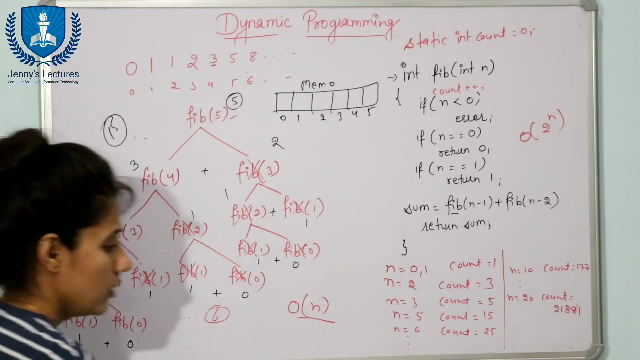 memoization technique, or you can say that dynamic programming approach, fine, so you just have to modify this code a little bit. how? how you will store these value? you will have to take one array, fine, or you just name of this array as memo: 0, 1, 2, 3, 4, 5, fifth index: fine. now when you will call, 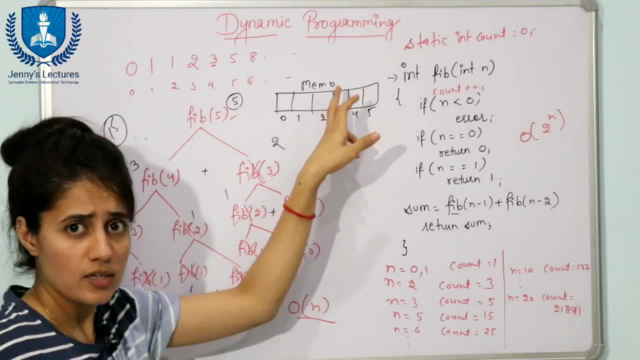 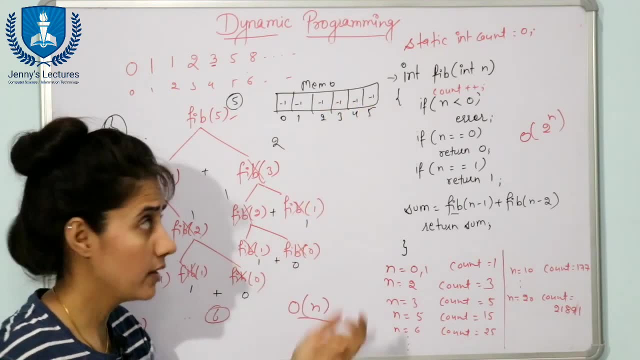 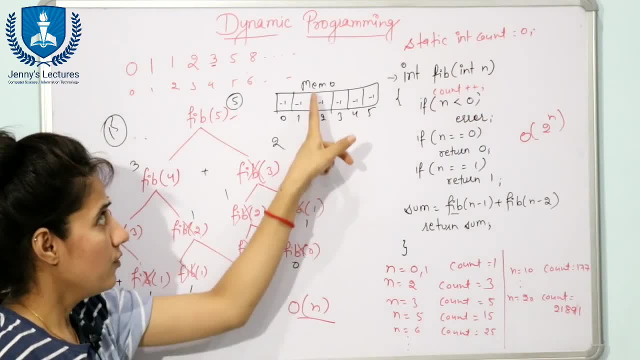 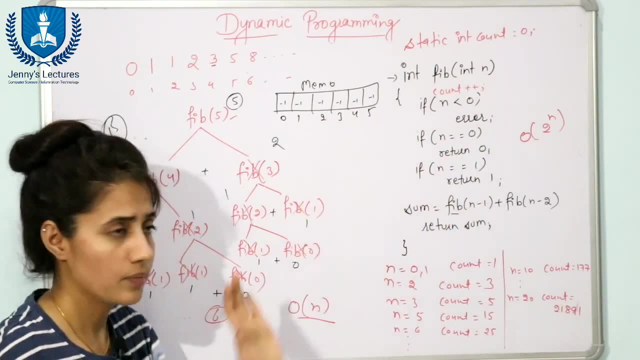 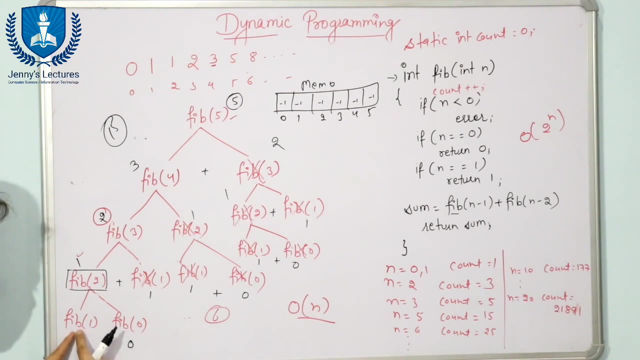 before this count plus plus, you will have to check if in this array, if value of that n is there, then you will return the memo value. otherwise you will call this function fine, like this, when we are calling this fib: one fine clue of 1. so in memo do we have see n, value is n, value is what. 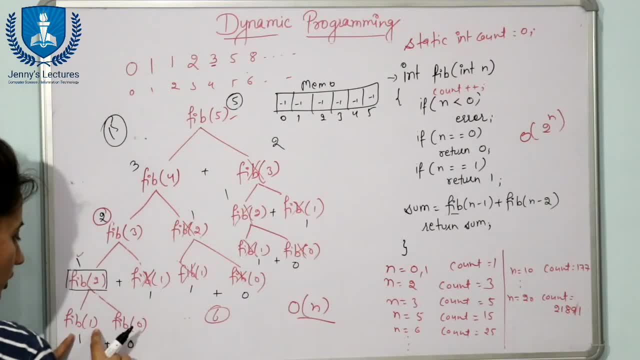 1.. so do we have something? no, this one is null, so we will call this one. we will call this function and for 1 it will return one. so here we will write one for 0. do we have in our memo? no, initially we don't have, so we have to call two rows. so after that it will return to zero füh. 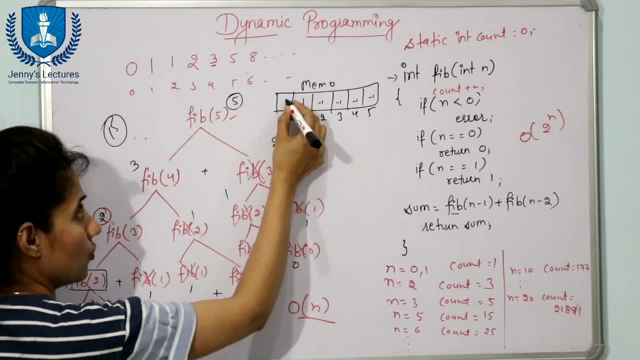 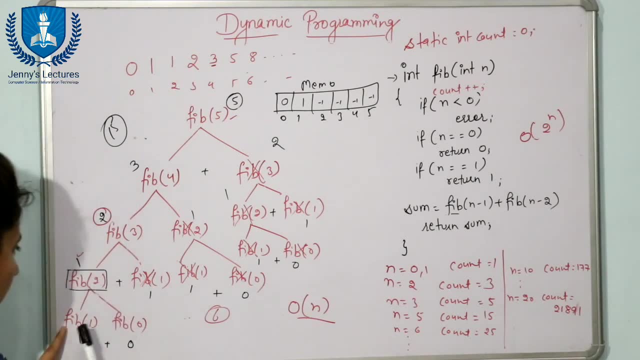 点 row we don't have, so we have to call, so after that it will return zero too, so we will store this 0 here. so that is why these are 2 function call 1 and 2. fine, now, 1 plus 0 is what 1? now this for fib: 2, n is 2, n is 2. this 1 value would be stored. fine, 3 function call 1, 2 and. 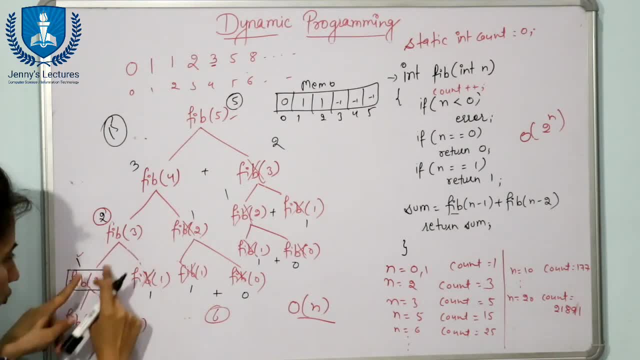 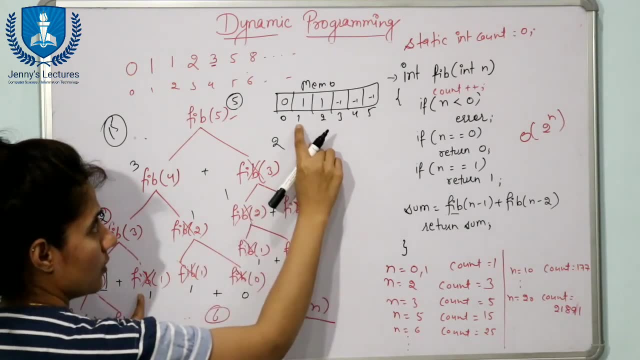 3. now see for this fib 3. we have to calculate fib 1, but do we have fib 1 value? n value is 1. check out: n value is 1. this is what memo of n. so n value is 1. memo of 1. yes, we have value we. 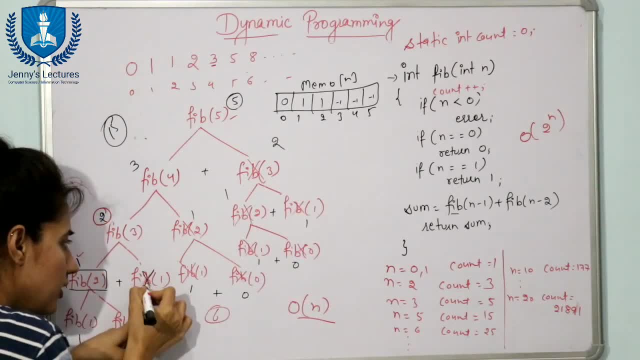 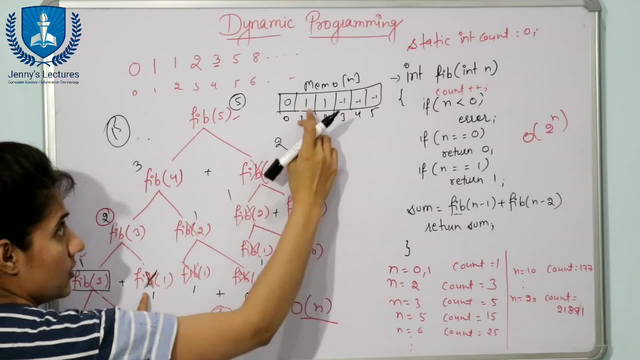 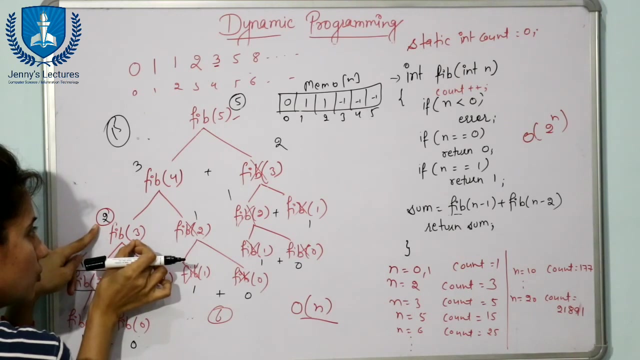 don't have null value. we have something, so no need to call this function, we just take this value. fine, so for fib 1, we simply take this value: 1 plus 1 is 2 and we will store this, this value. we will store this value. fib of 3 to here only fib of 3: n is equal to 3, n is equal to 3 here. 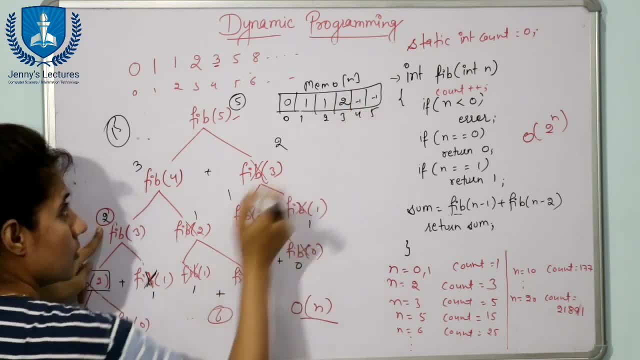 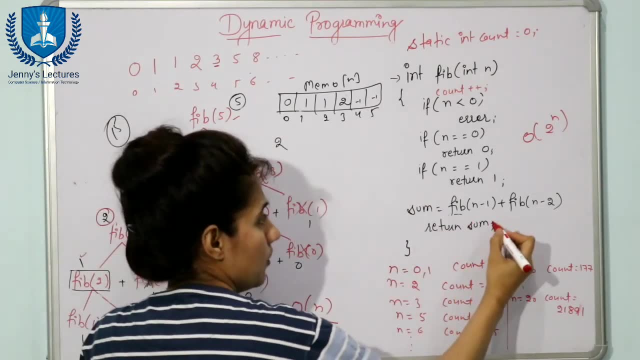 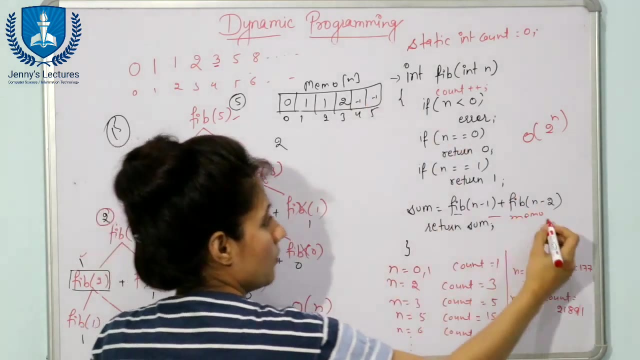 here, then we will store here 2. fine, now how you will store this value, say, you have to modify this code a little bit before returning this sum. simply, maybe you have to write something like this: if you are taking memo, then you have to write: memo of n is equal to. 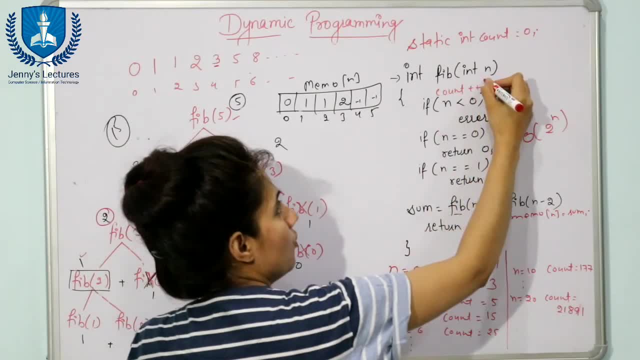 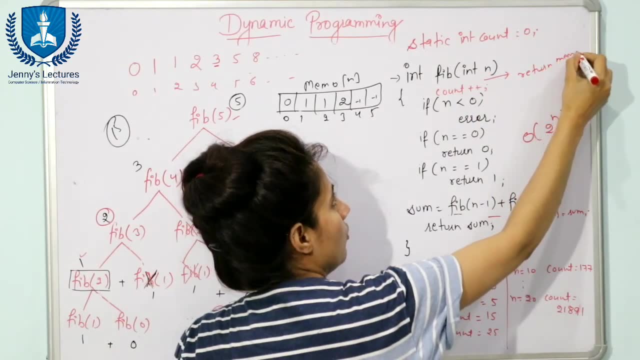 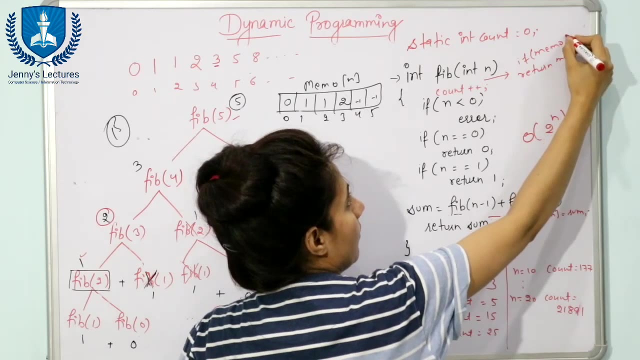 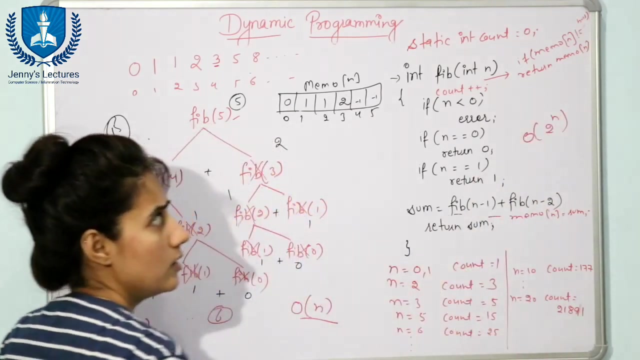 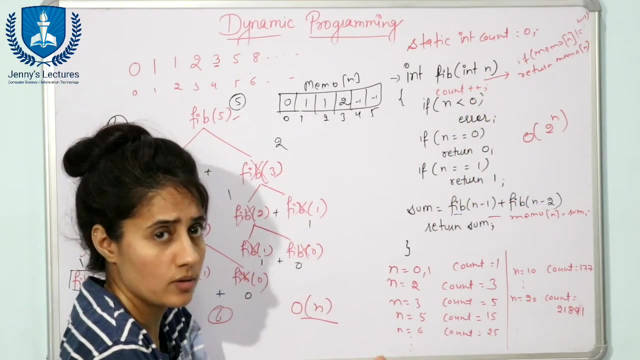 sum. you have to store this value and before this count plus plus, you have to return value. also, it is equal to to value sign. you have to check if, if memo of n not equal to null, then only you will return this memory, something like this: I'm not saying that this one is the correct. you have to write. 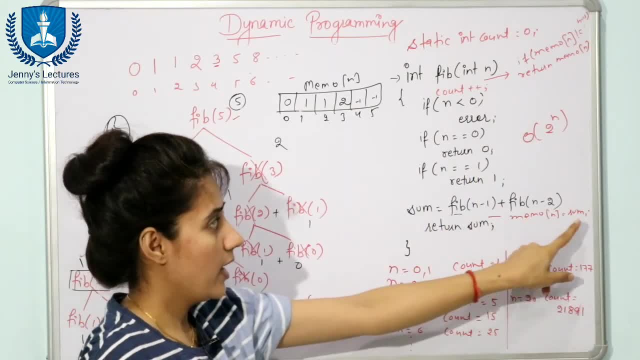 down exactly the same. but you have to implement this logic. before this count plus plus, you have to check if we have value for that end in the memo. then you have to return that anymore and before returning this sum, we will add, we will store the sum value to this memo array. fine, 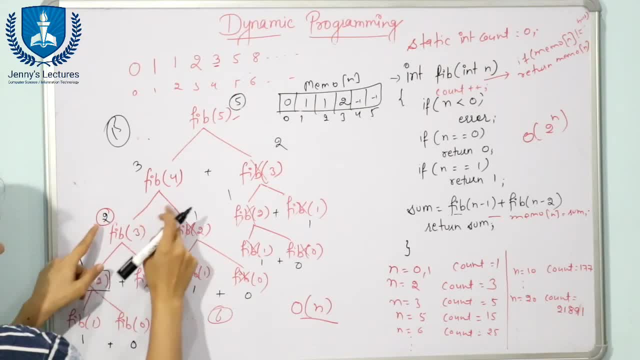 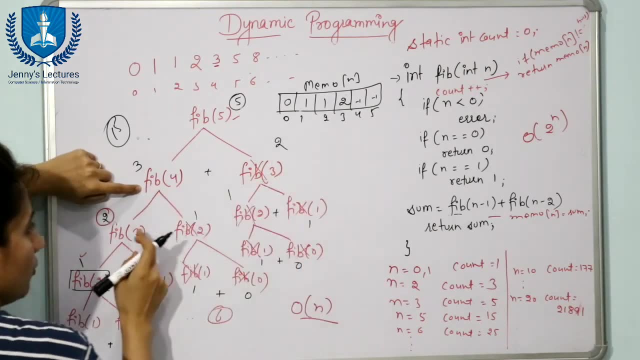 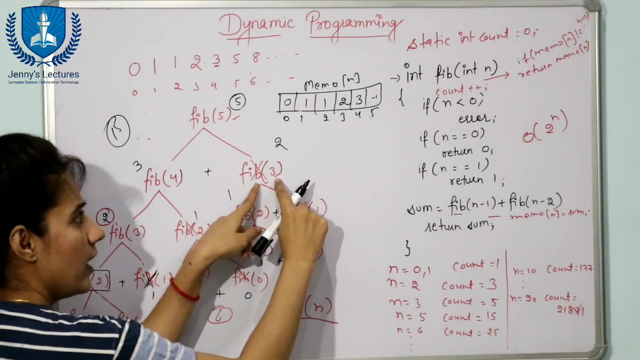 something like this: so now see now for fib. see for this one, this one, we have this: 2 plus 1 is 3. now we will store at fib 4. see here we will store what 3. fine, now check out, we have to calculate this one. but for this we have to calculate this value, fib of 3. now do we have in memo array for: 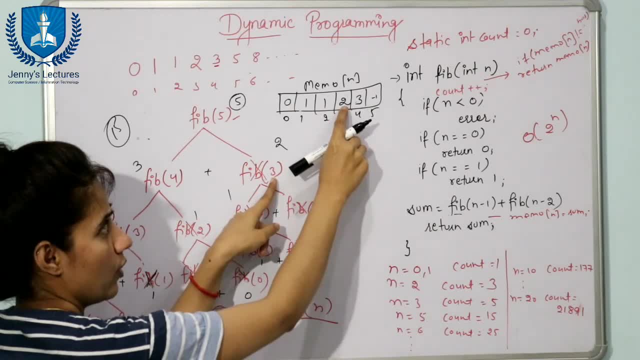 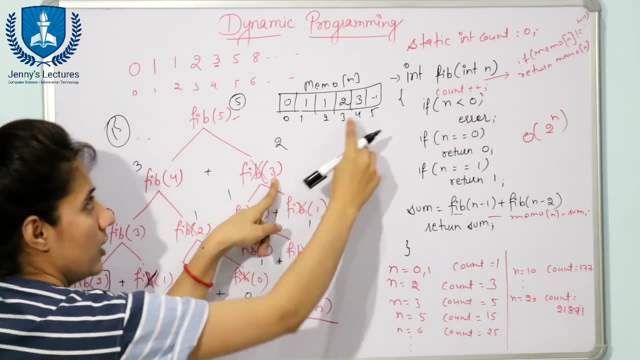 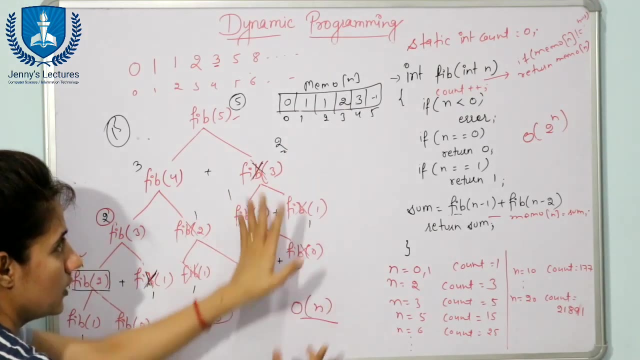 this value fib of 3, see n value is 3, n value is 3. do we have value? yes, this one is not null. that is why i am saying not null. then you will return memo, then you will return what this 2 value, this 2 would be returned and we will not call this one and we will not call this 3 we. 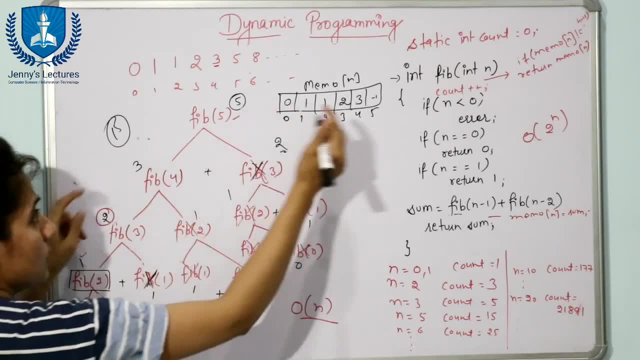 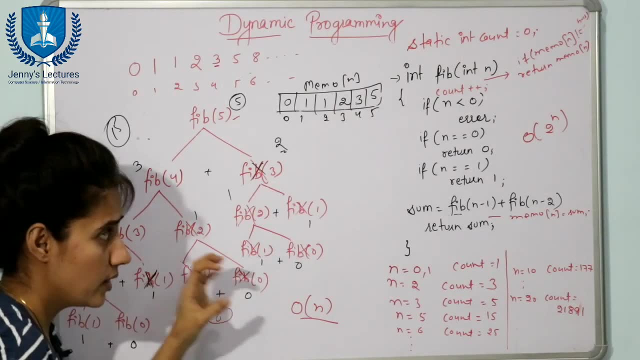 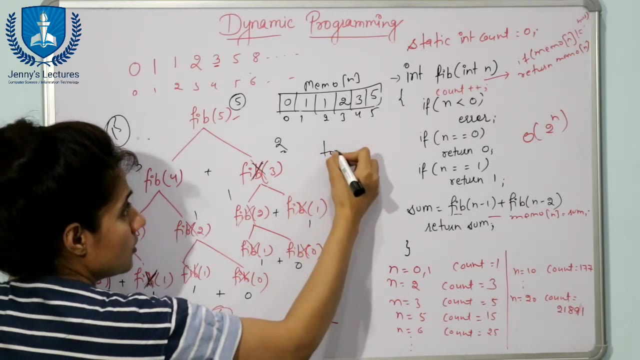 will not generate this tree. fine, so 3 plus 2 is 5, simply 40: 3. we will put 5 here and the answer would be 5. so this is, this is how, using the memoization technique, you will avoid the function calls, and this is what this is known as top down approach. 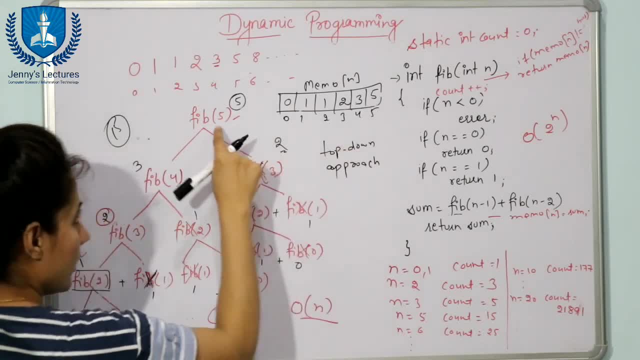 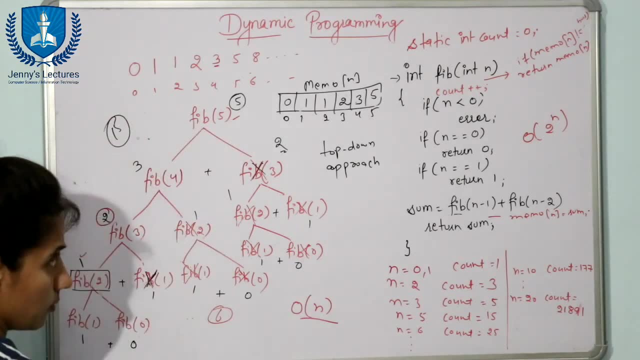 why top down? because we are going to start from here only and we are going to divide this problem into sub problems, sub problems and then finally we are obtaining the result of this problem. so this is top to down approach. so in this technique also we are using what 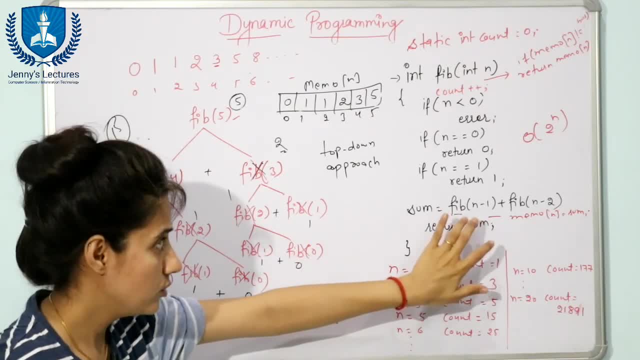 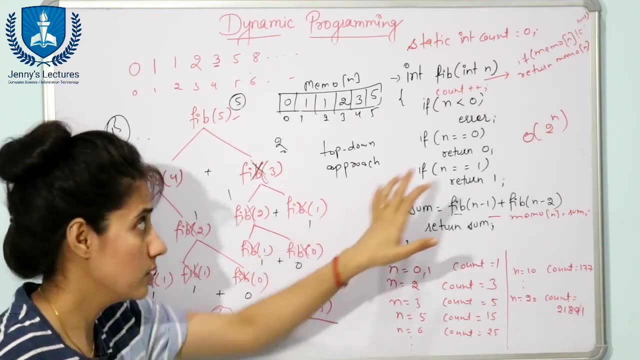 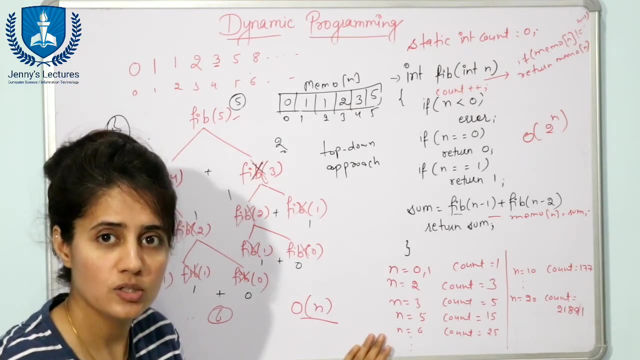 60 recursion. but we have just modified this recursion, we have just added one simple logic, extra logic, to store the intermediate results. fine, so this is known as memoization technique, or you can say this is known as top-down approach. now next is bottom-up approach, or you can say that tabulation. 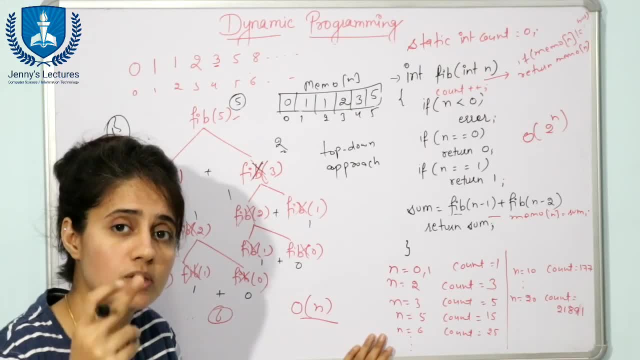 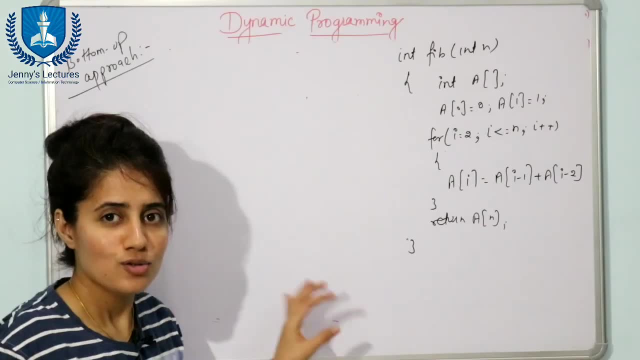 method. so basically, when we implement dynamic programming, then we will, then we use that tabulation method, we don't use this top-down approach, or you can say memoization technique. so now we will see what is that bottom-up approach. see, in this case, what we are using. 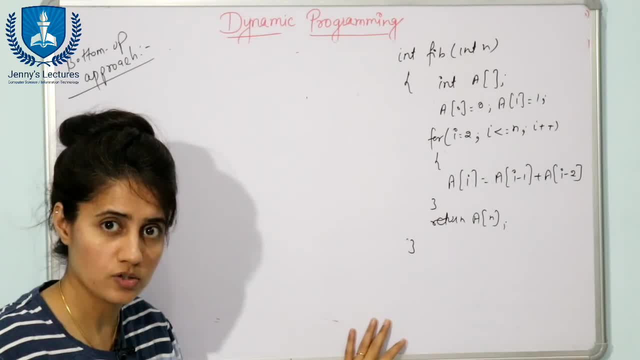 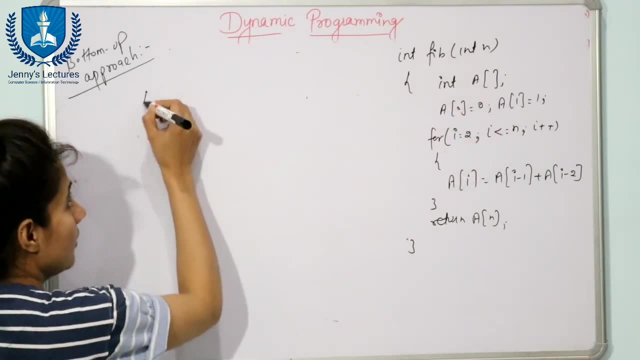 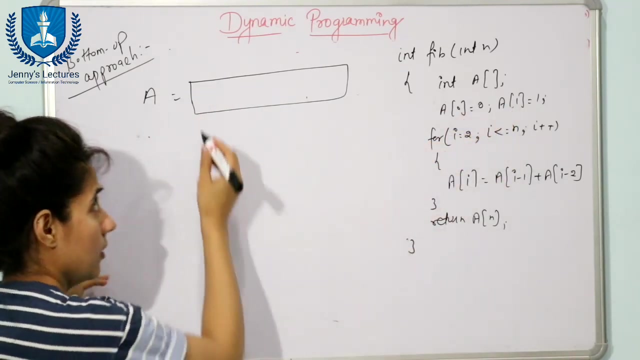 iterative functions we are using, rather than that recursive function- fine, and we will start from the bottom only so same function is there. we have just taken one array, fine, and array of 0 and array of 1, array of 0 and array of 1. we have initialized because starting 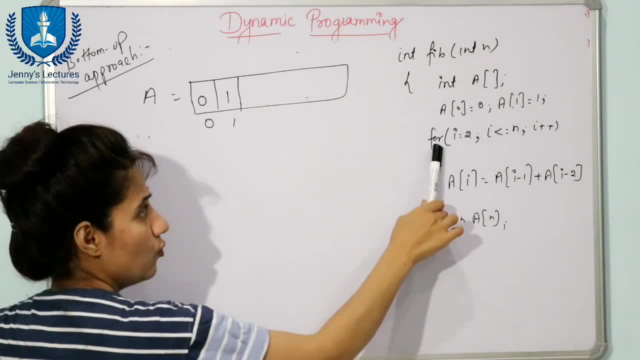 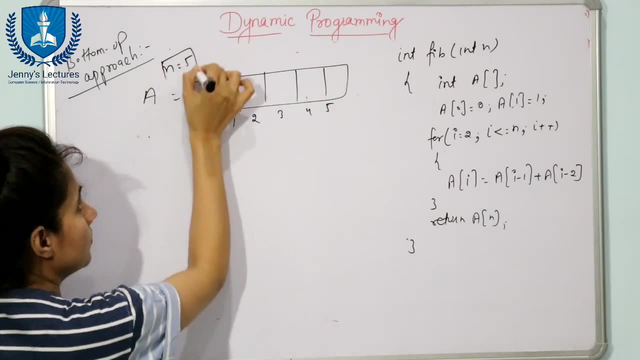 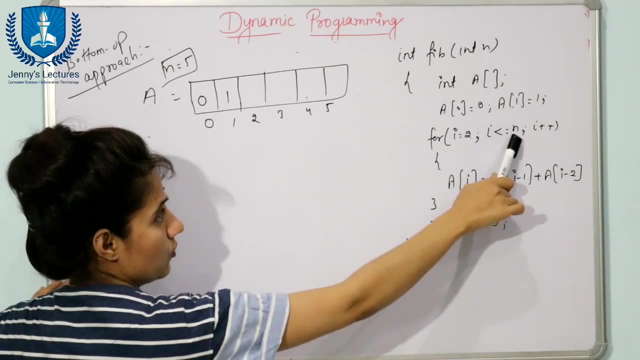 value we have. that would be 0 and 1, 1, and then loop would be started from this. 2 when n value is 5. okay, so i is equal to 2, i is equal to 2 and i should be less than equal to 10. n is equal to 5. yes, this one is true. so if this: 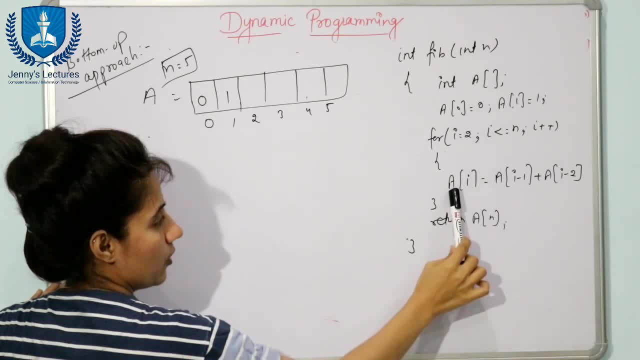 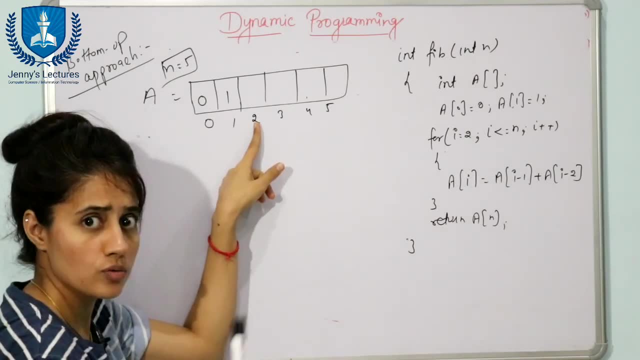 condition is true, then control will go to within this loop. now, a of i, a of i means a of 2, a of 2 is what? a of i minus 1 plus a of i minus 2? same function. i minus 1 is this one, i minus 2 is this: 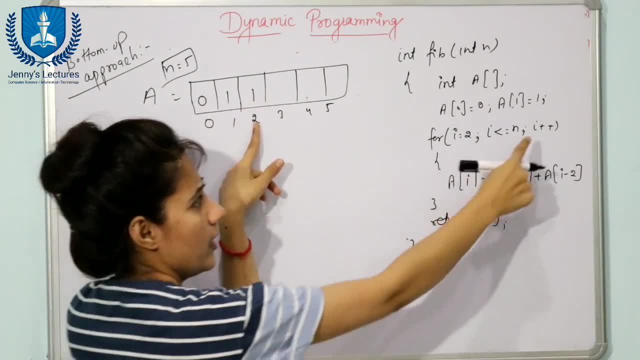 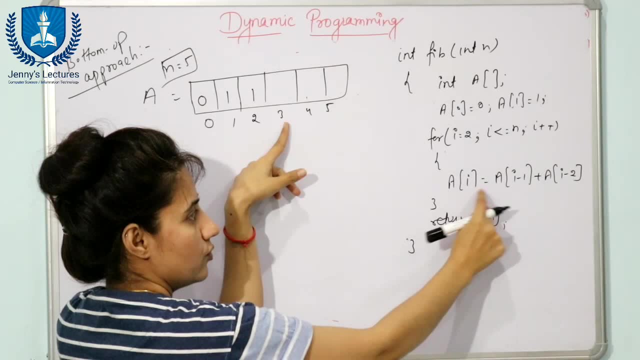 one. so 1 plus 0 is what? 1, now i plus plus now i value is what 3, 3 is less than 5. yes, control will go within this loop. a of 3 is equal to 3 minus 1. 3 minus 2 means this: 1 plus 1, it would be 2. 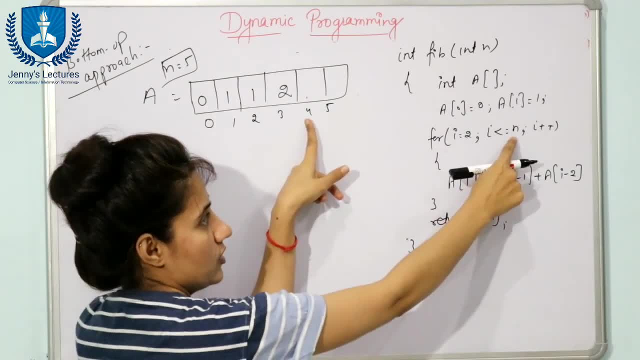 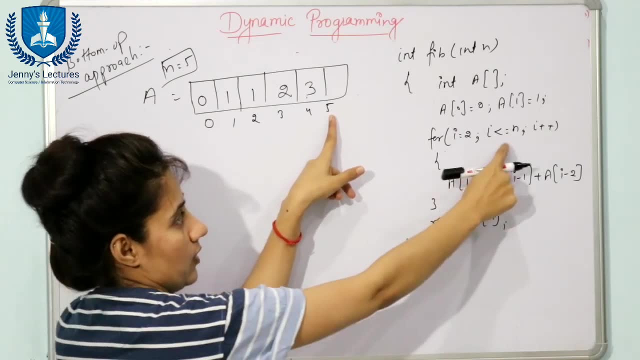 again: i plus plus i is now 4. 4 is less than equal to 5. yes, within this loop. then we let 2 plus 1 is 3, now i is equal to 5. 5 is less than equal to n. yes, n is 5. so we will do what 3 plus this one is. 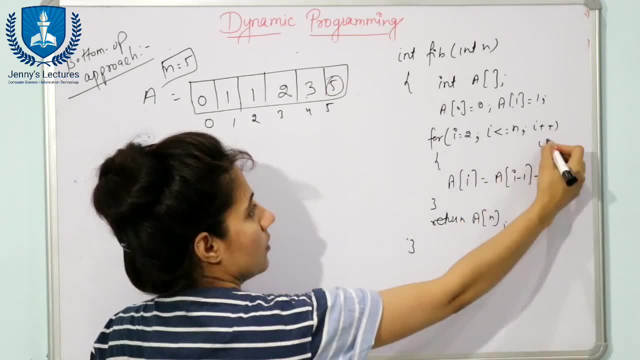 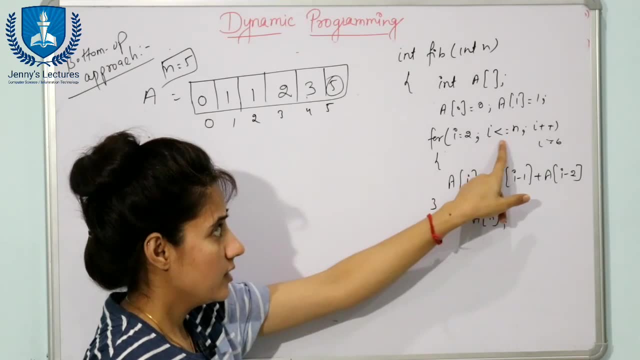 5. now again i is equal. i is equal to now 6, but 6 is not less than equal to 10, so condition is not true. but 6 is not less than equal to this n. n is 5, so condition is not true. then control will go. 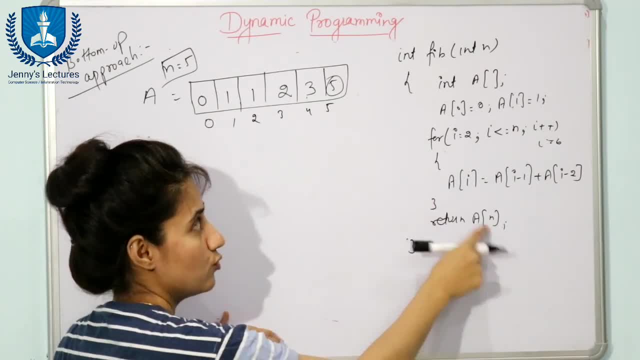 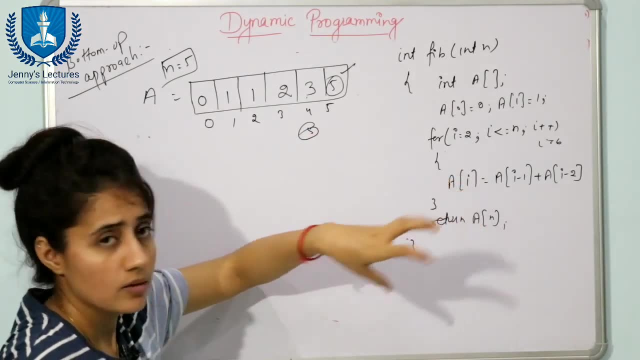 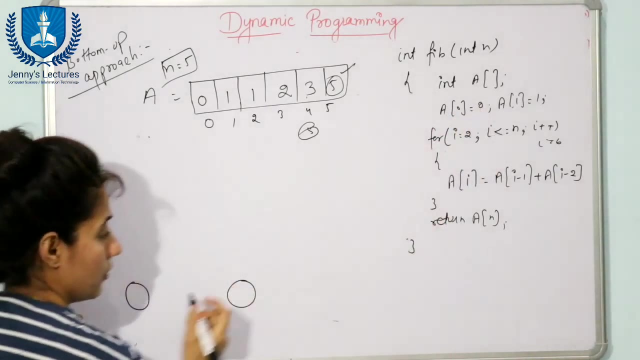 from out from this loop and return a of n? n value is 5, we will turn a of 5. that would be 5.. fine, so here we are, starting from the bottom. only see here we have for a of 0, we have 0 value and